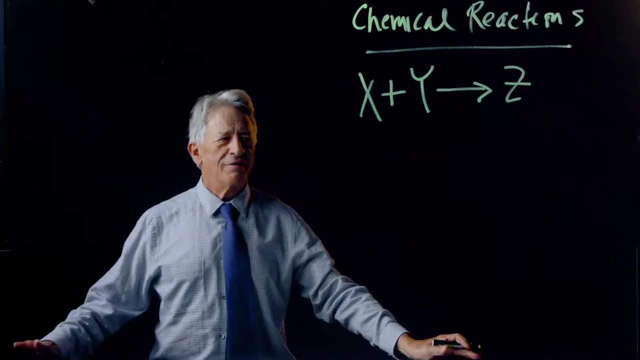 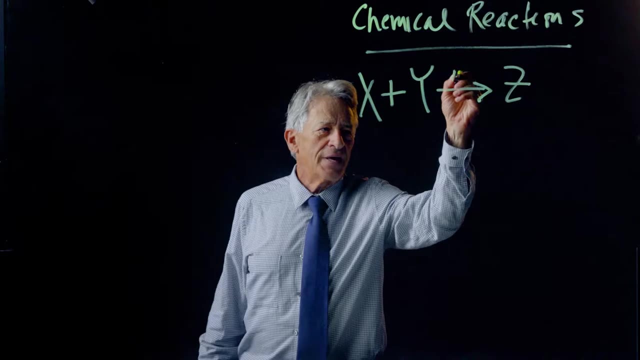 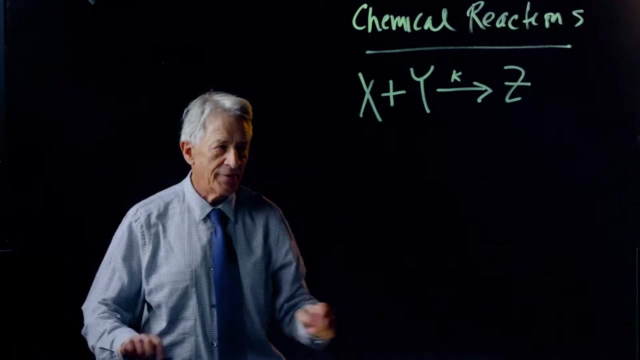 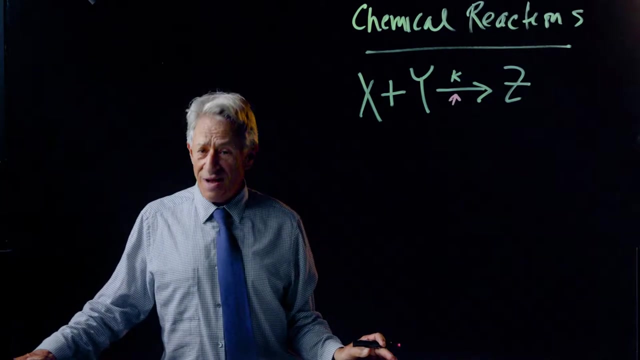 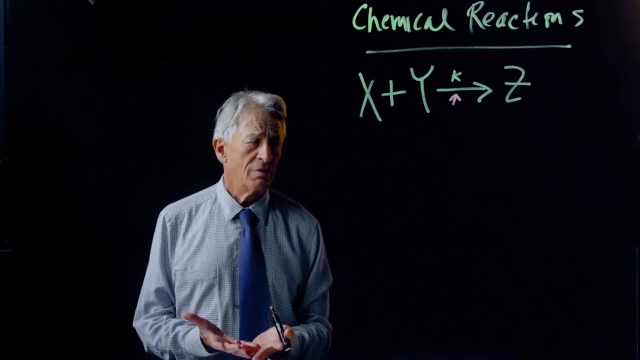 this And that's read: x plus y goes to z, And sometimes there's a little k up there. Now, what does that mean? First of all, the thing that we have to emphasize is that that goes to arrow is not a mathematical symbol. It's standing for a physical, chemical reaction. 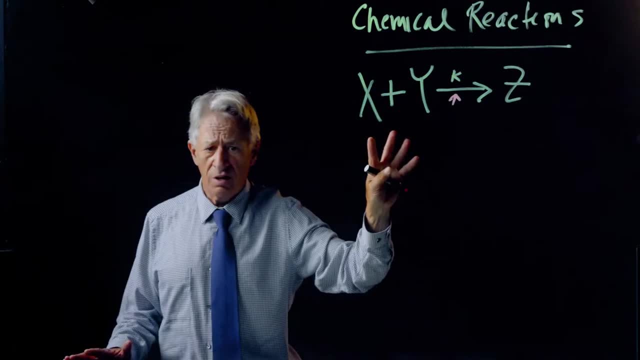 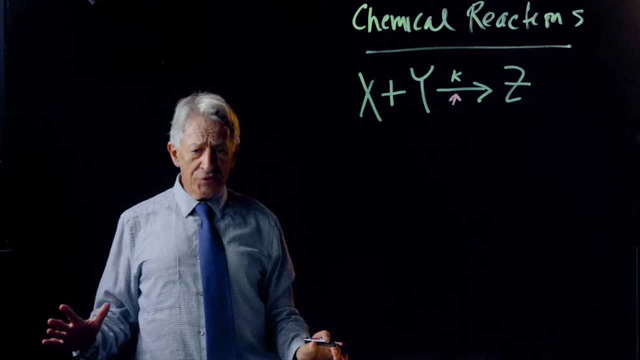 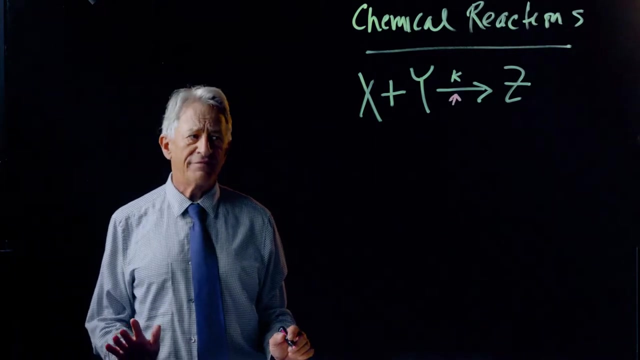 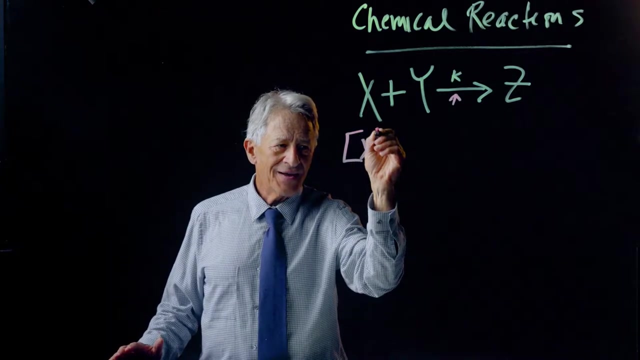 So we have to turn this rate law into a differential equation. So how do we do that? Well, the first thing that we have to do is we have to decide what our state variables are. In this case, we're going to take as our state variable the concentration of x: the concentration. of y and the concentration of z. This looks like this one here. One point is to the left. So first of all, I want to clear all these things by Iran termination. This looks like this is right here, And what we'll need to do now is to take and kung letters to make a. schwieriest one here for our noise general of x and my noise general Also. I want to make this coeval, introduce a規 as the maximum, but then we're going to have certificate things And once you represent these właśnie, and so on, and so it's there. This is now what I'm organization. 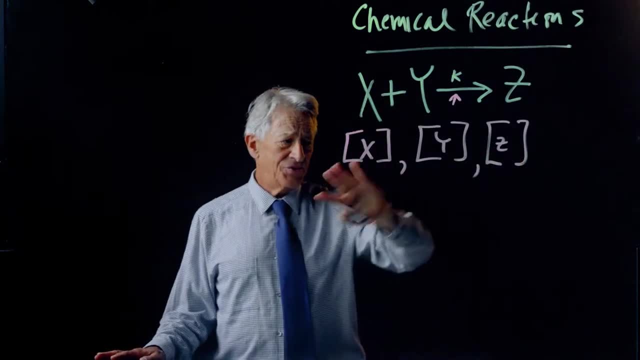 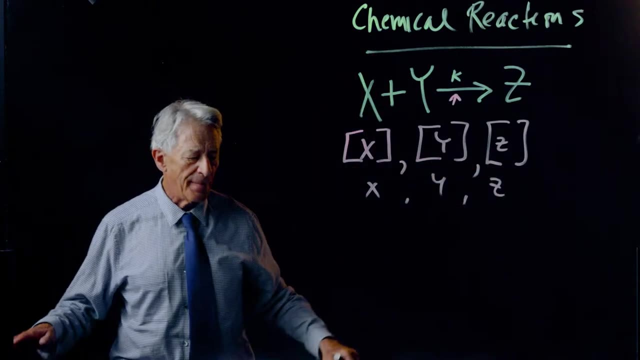 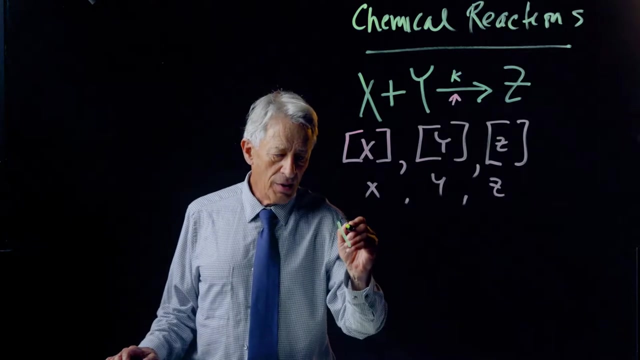 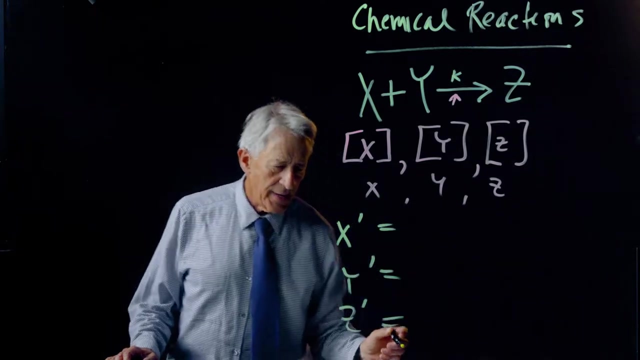 concentration of z and to get rid of those- I'm just going to call those variables- x, y and z standing for their concentrations. Good, Now the next question, as we make a differential equations model, is: we put down our x prime and our y prime and our z prime and we ask what makes x go up? 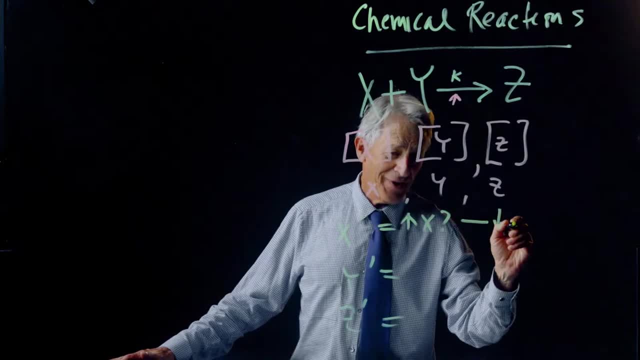 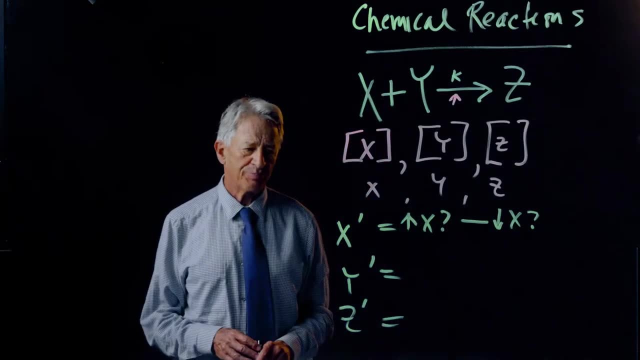 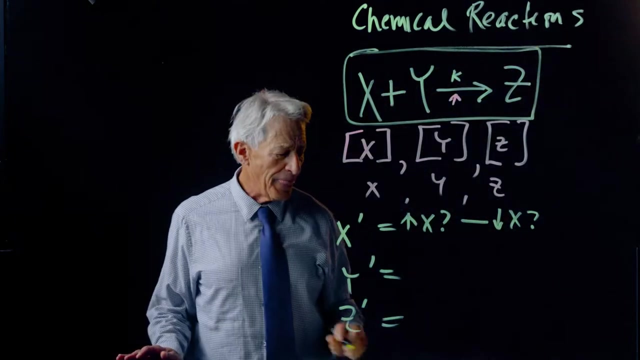 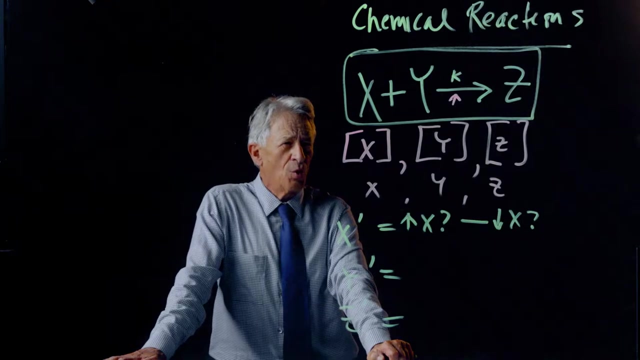 And we subtract from that whatever makes x go down, and, of course, the same thing for y and the same thing for z. Now let's stare at this equation- not equation, excuse me- this rate law- and let's ask ourselves, in this rate reaction, what makes x go up. 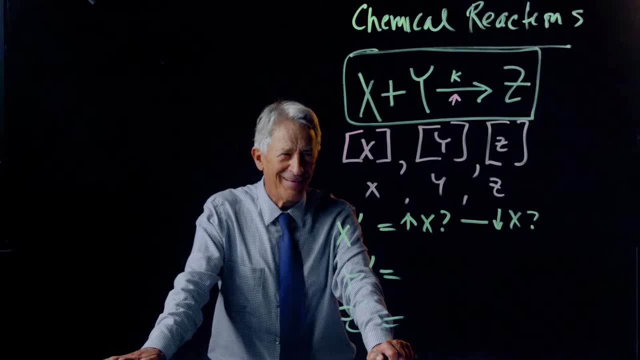 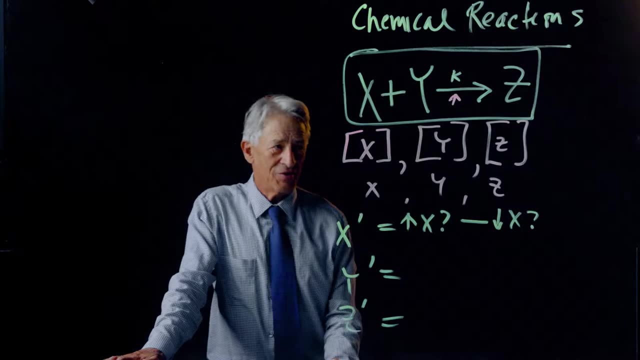 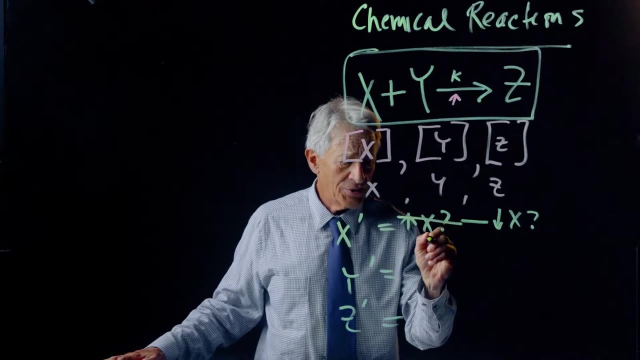 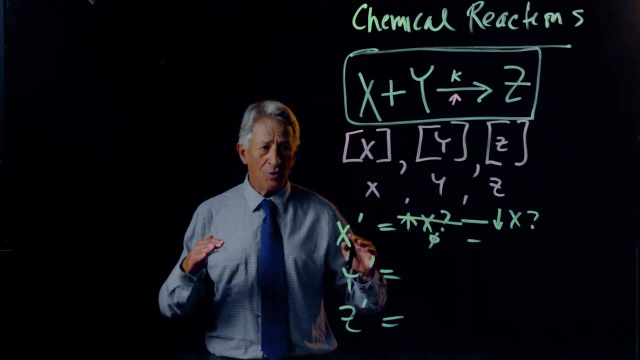 And we'll see, And we'll see, And the answer is nothing. As written here, there is no arrow going into x, and because there's no arrow going into x, nothing makes x go up, and so that quantity is zero. Now the next question is: what makes x go down? and the answer is: 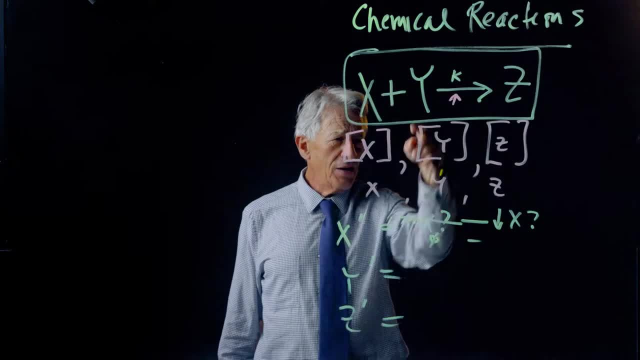 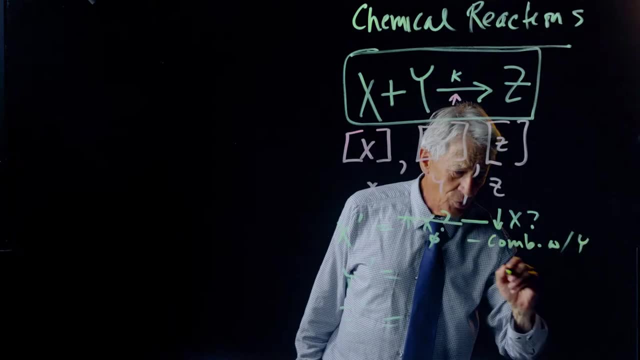 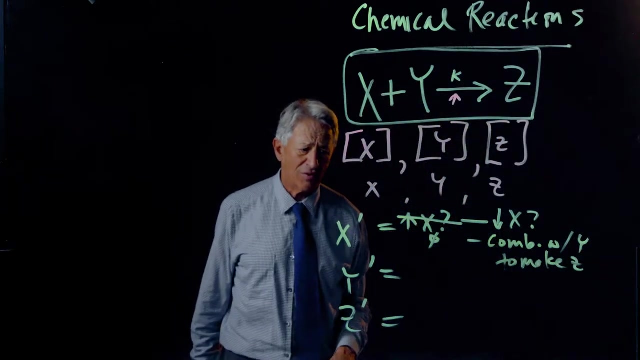 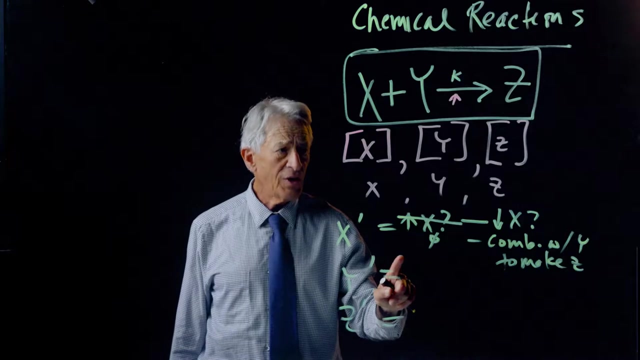 combination with y to make a z, And I'm just going to write that in English. Combination with y to make z. We're going to have to figure out what that is mathematically. What makes y go up? Again, nothing. What makes y go down? Combination with x to make z. 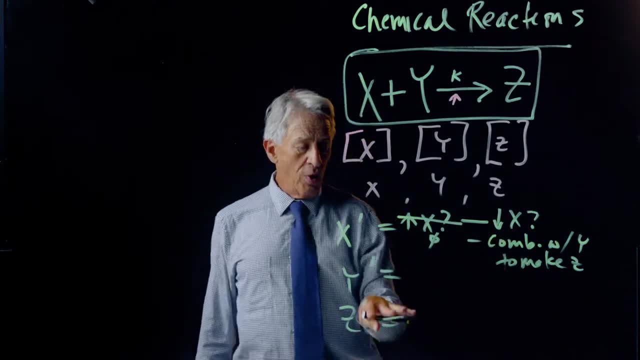 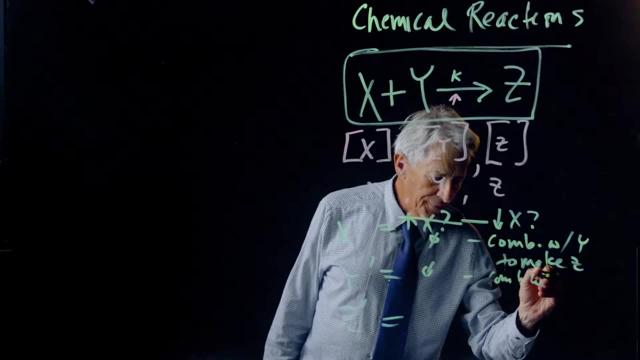 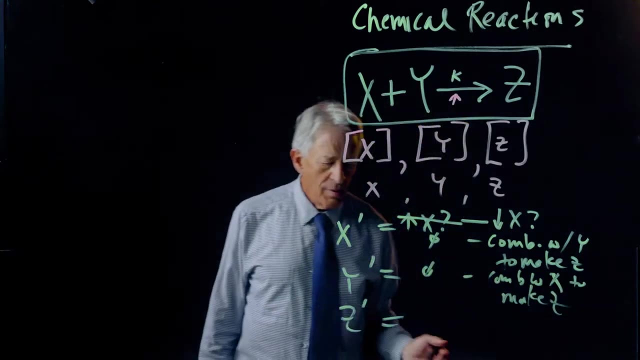 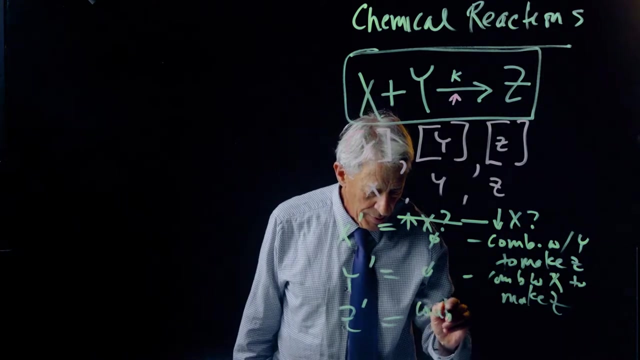 football? similarly, What makes z go up? So let's just put that Nothing, and then combination with x to make z. and then what makes z go up is the x's and the y's, combining combination of x and y. and what makes z go down is: 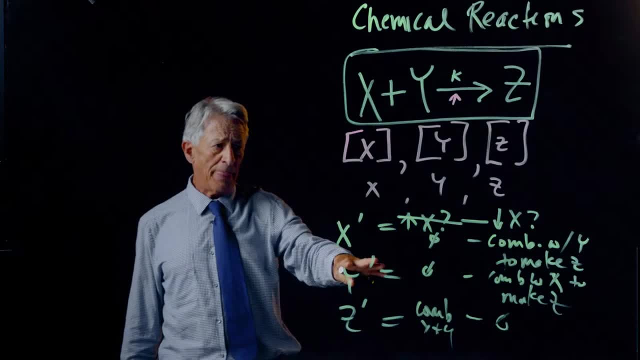 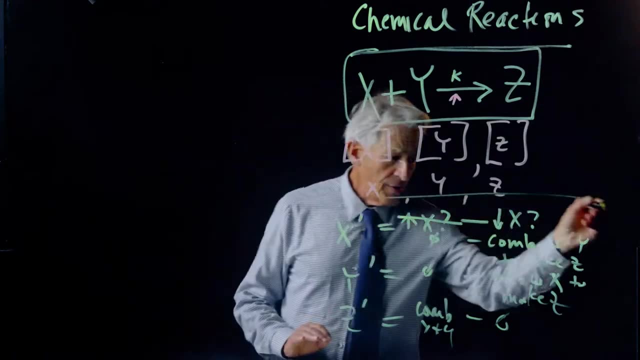 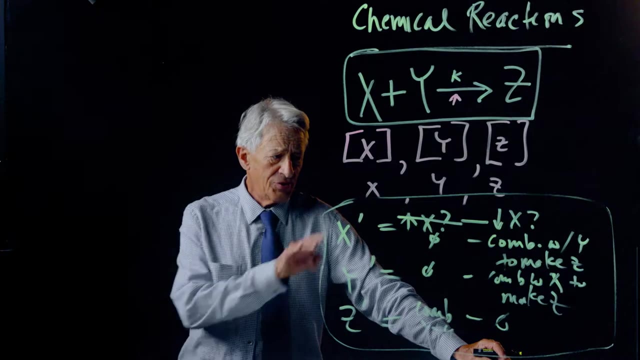 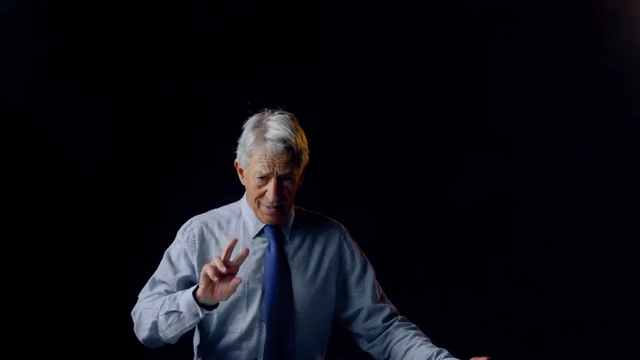 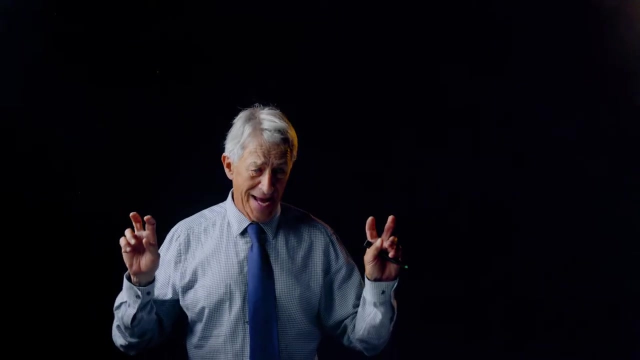 nothing in this reaction. So we've at least put in words here to represent our differential equation. Now we have to figure out some math to express that combination term. So in order to turn that combination of x and y, or x meets y, and you may remember, 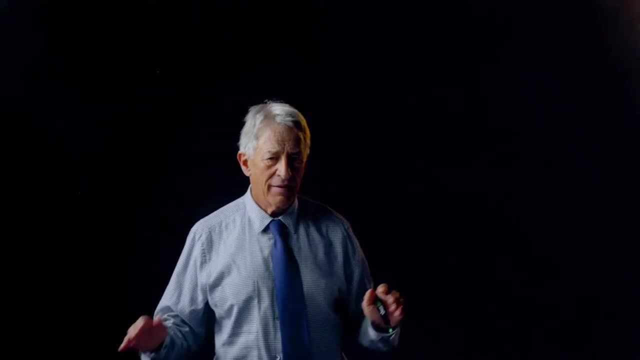 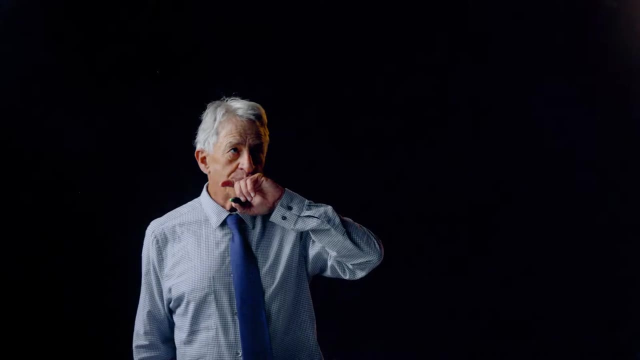 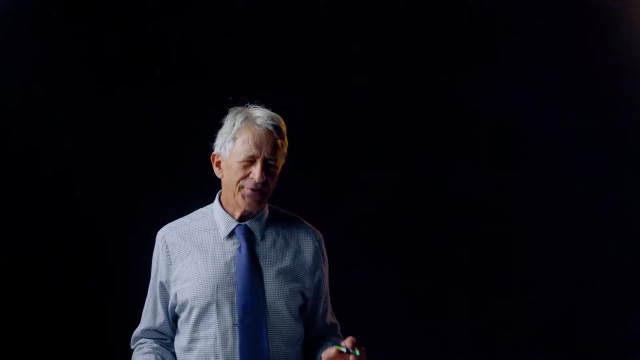 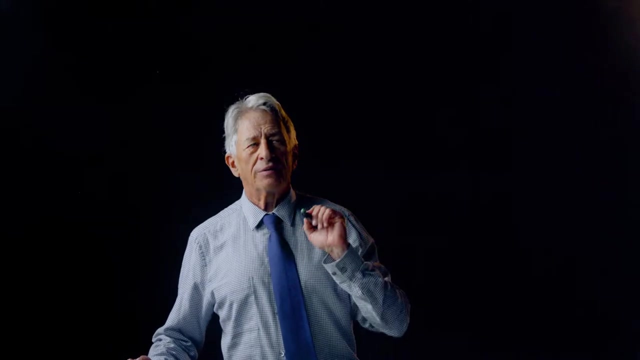 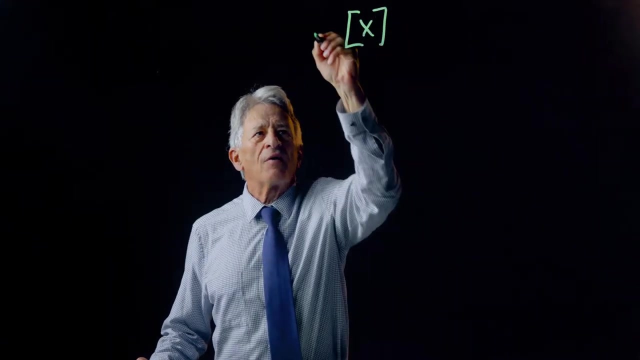 that from Sharpe-Tuna, x meets y. how can we quantify that? So the first thing we need to do is we need to understand that the argument that we are going to make is essentially an argument using probability. So the first point, the first observation I want to make: we said the variable x stands. 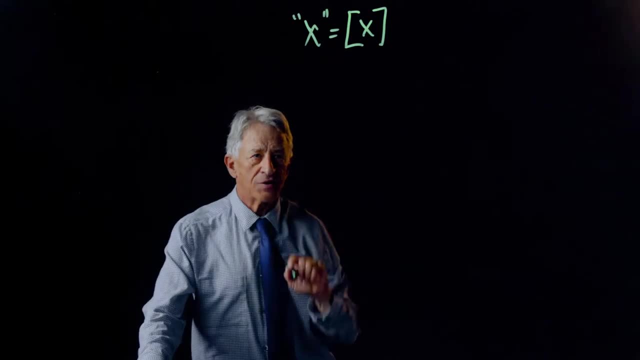 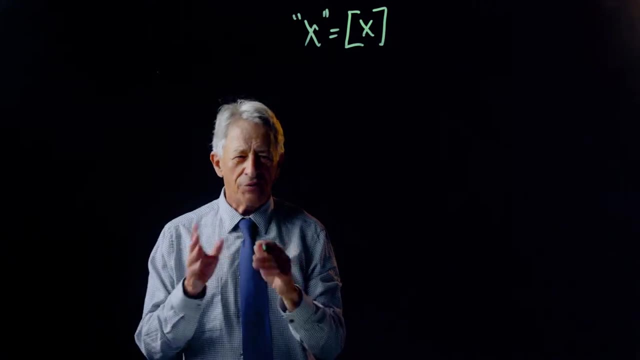 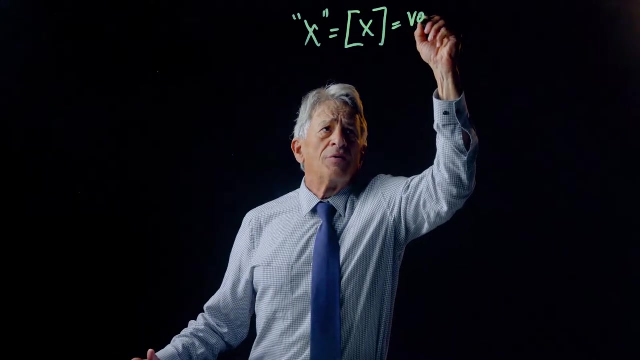 for the concentration of x. I want to stress that what we are talking about with those square brackets, it's not the molarity, the usual concept of molar concentration, of the atomic weight and stuff like that. this is what is called the volume concentration in chemistry, and it is simply how much here. 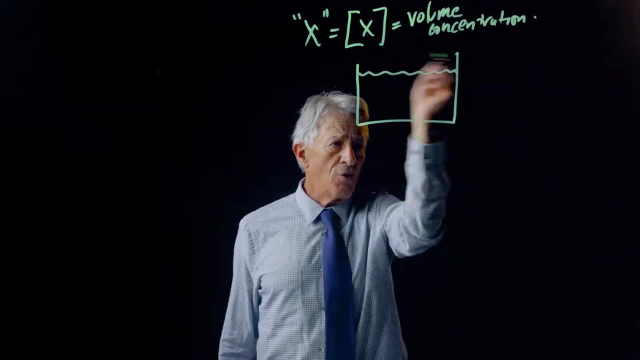 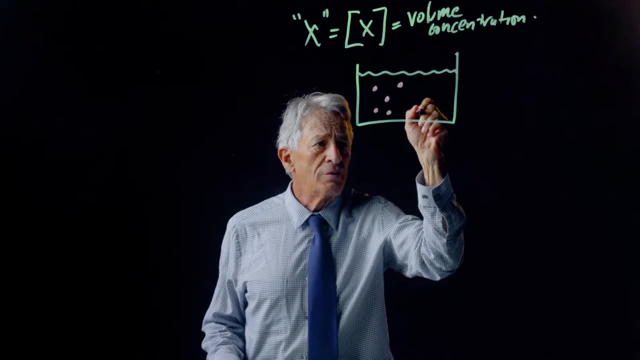 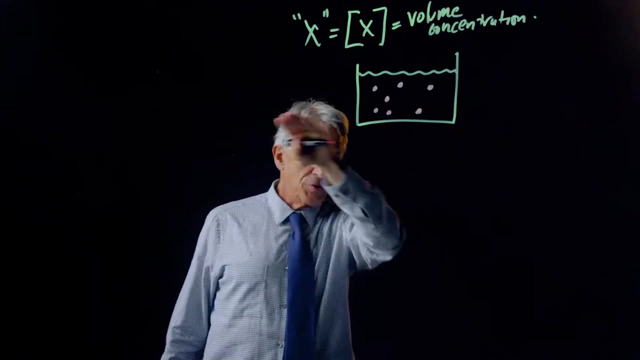 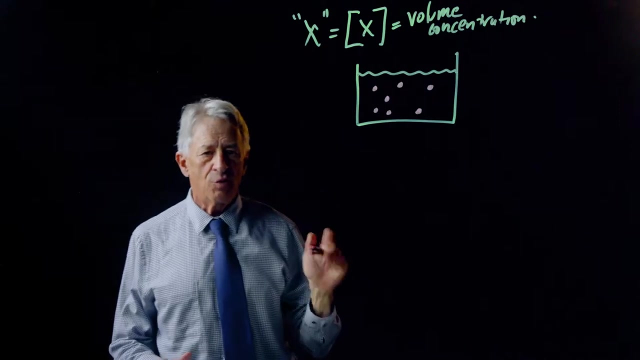 is your beaker, and here is the whole volume, v, and here are the x molecules and here is the volume concentration of x. and the question is: what is the volume of the pink dots divided by the volume of the beaker? That is the volume concentration of x and it is what we are using as the variable. 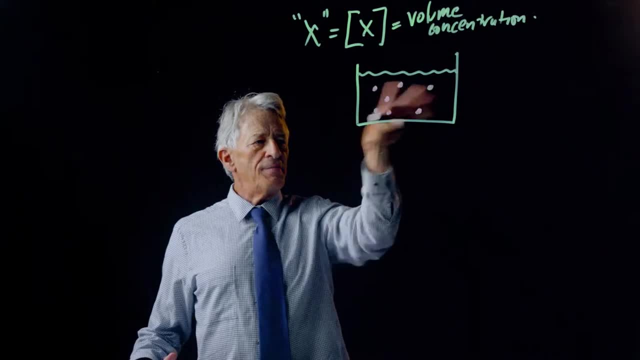 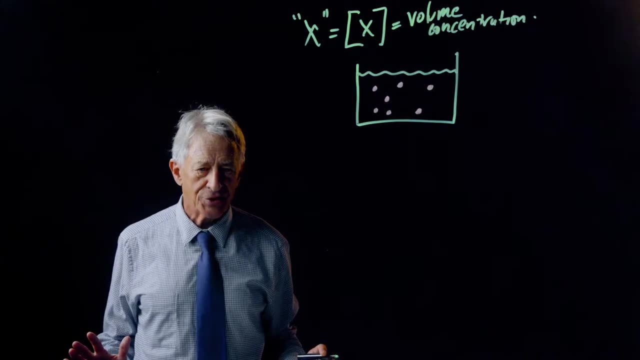 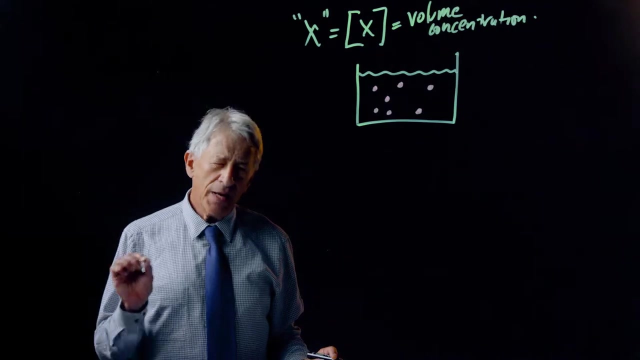 Now here is the key point. You see some pink dots in the black background and that the ratio of the pink to the black is the volume concentration, or rather, the ratio of the pink to the whole thing, That is the volume concentration. And now I want to ask a question. 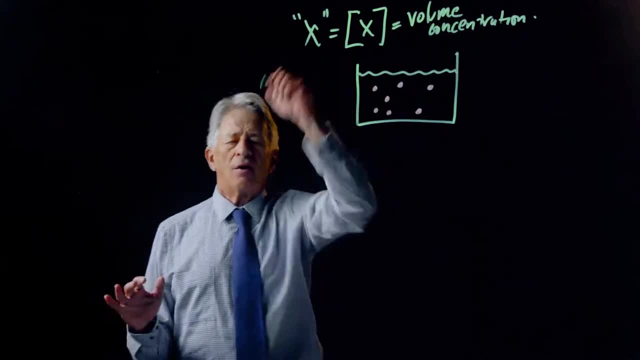 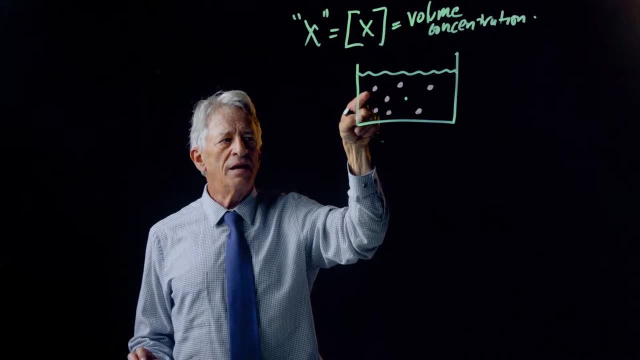 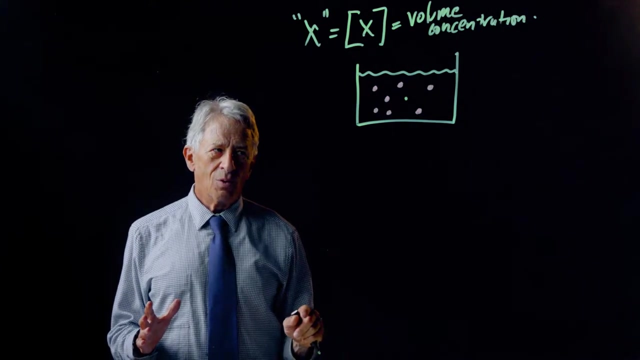 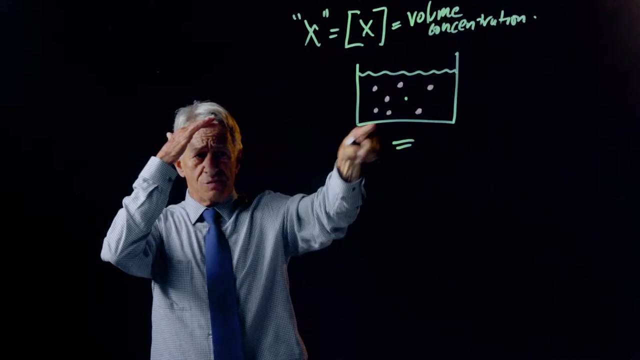 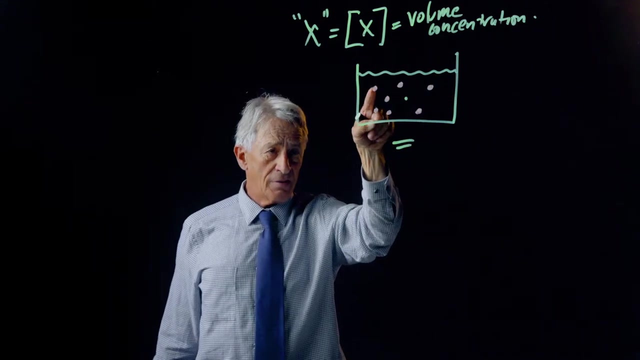 What is the probability that a random point chosen in the volume will contain an x molecule? What is that probability? Well, it is obvious. The probability equals the volume concentration. If I am just blindly picking a point here and one quarter of the points here are occupied, 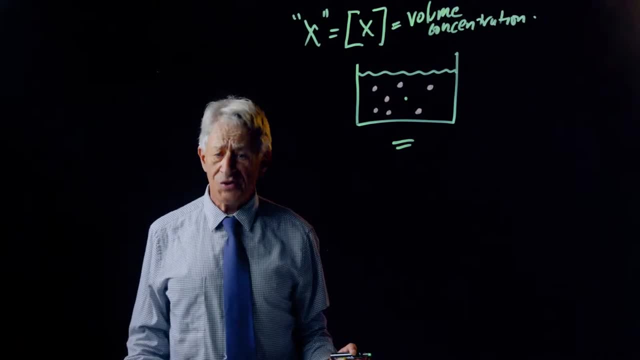 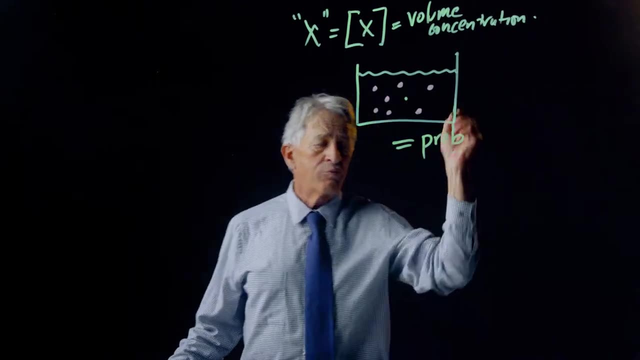 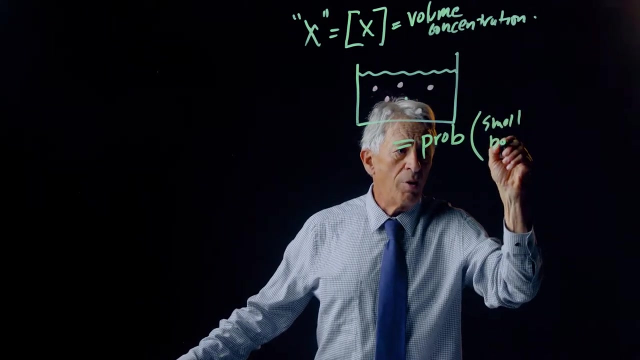 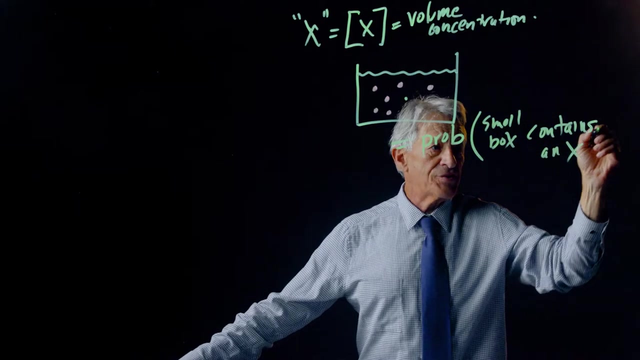 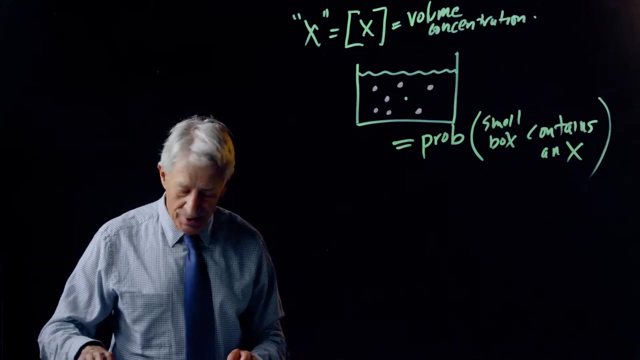 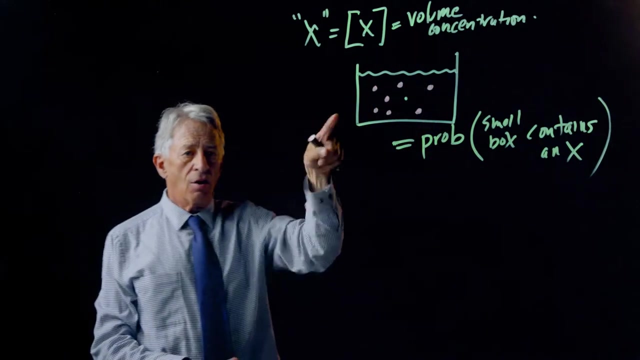 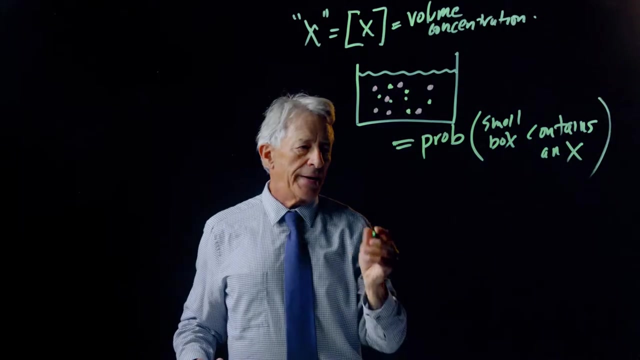 by red dots, then the probability of picking a red dot is 25%. So this is equal to the probability that a small box contains an x. Now let us ask ourselves what is the probability of finding a y molecule? Well, here are the y molecules. 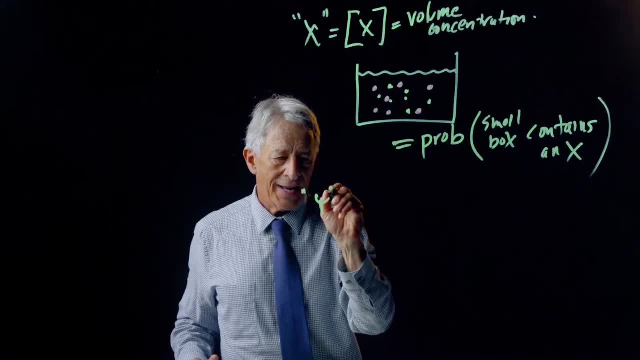 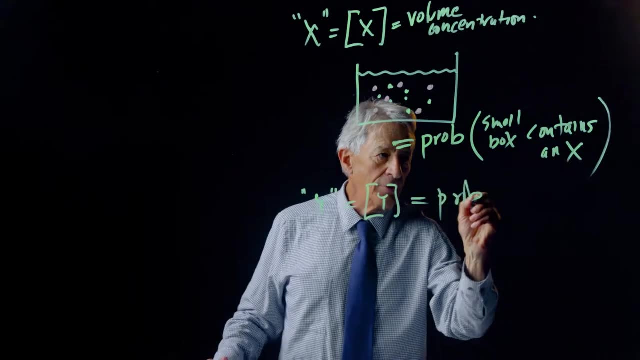 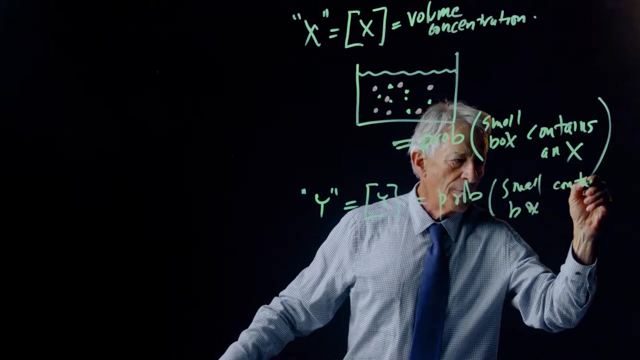 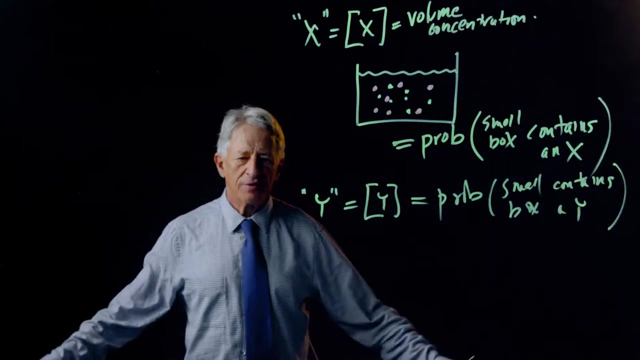 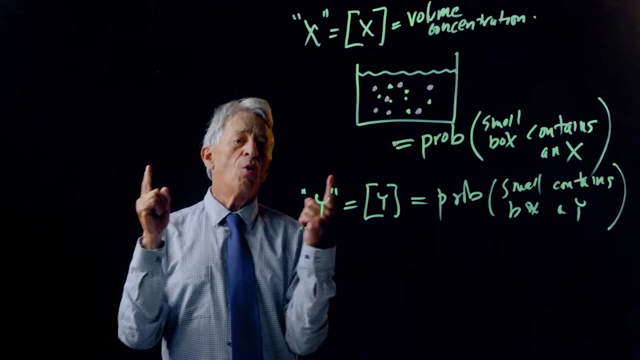 It is obvious that the variable y contains a potential s of x, which is the volume concentration of y is equal to the probability that a small box contains y, contains a y. Now it's very easy to ask the question: what is the probability of an x meeting a y? 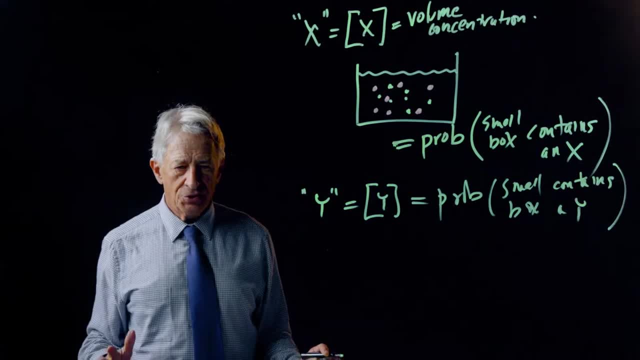 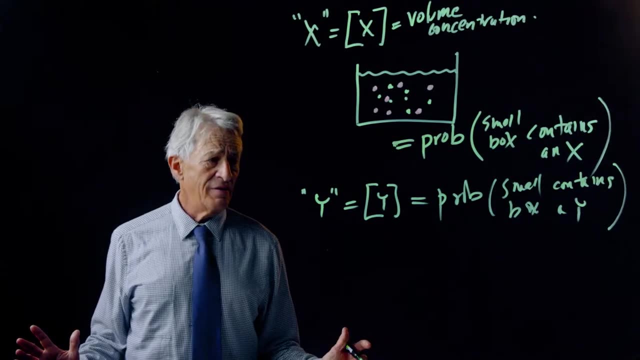 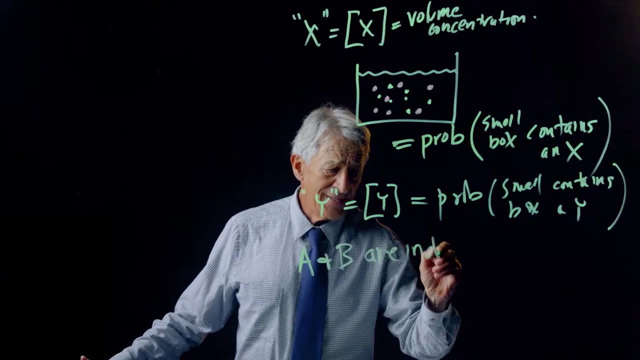 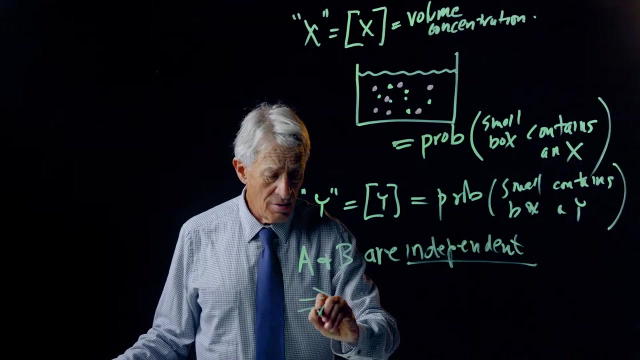 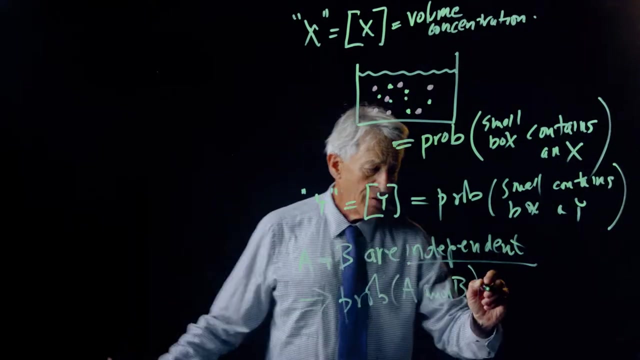 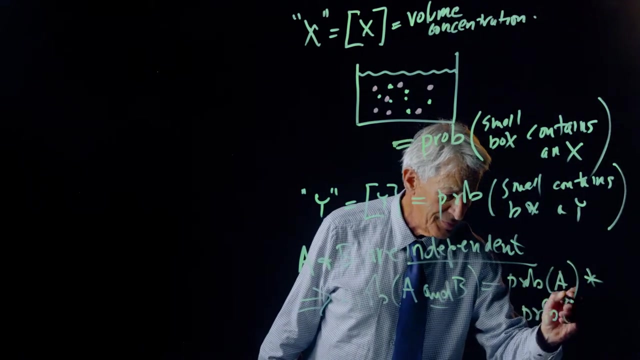 And in order to answer that, we go back to a very basic principle of probability theory, which says that if a and b are independent, then the probability of a and b and b is equal to the probability of a times the probability of b. 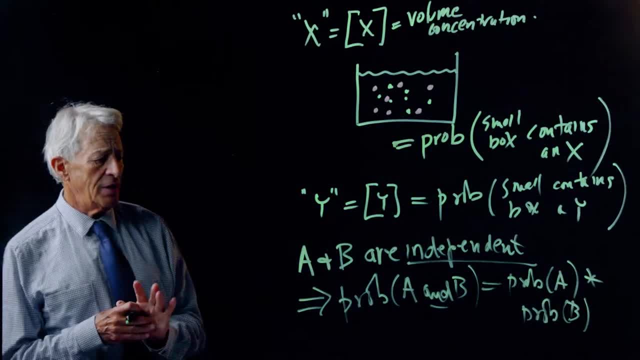 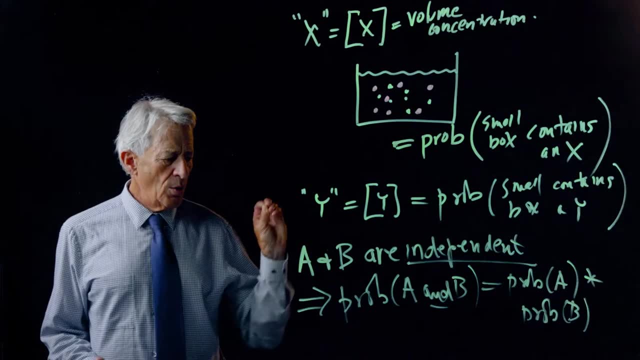 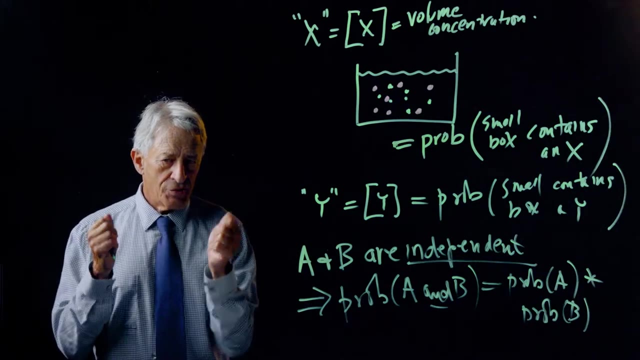 So, for example, the probability of drawing a red queen from a poker deck, that's probably. you have to draw a red card and a queen. So, first of all, is redness and and queen-ness independent? Yes, they are. 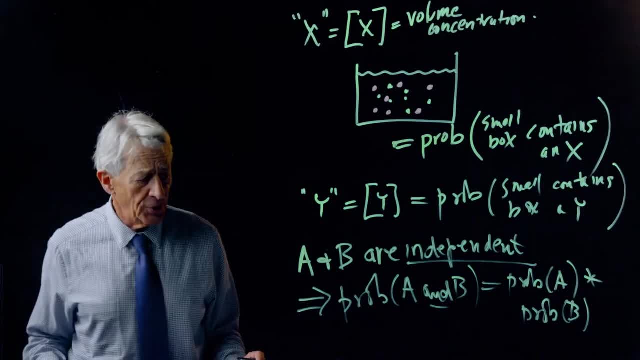 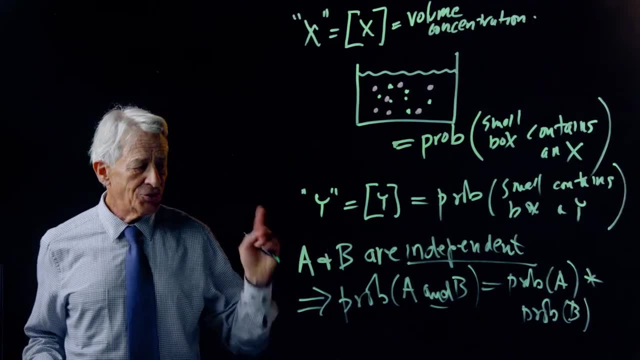 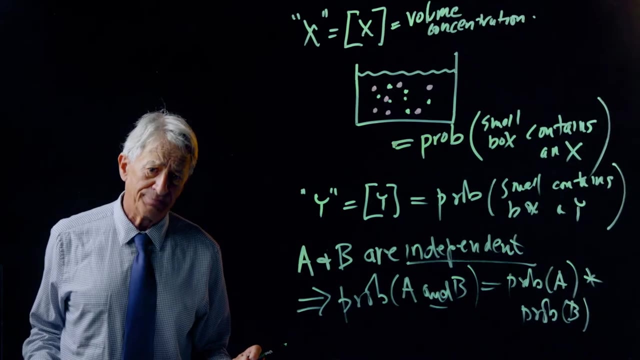 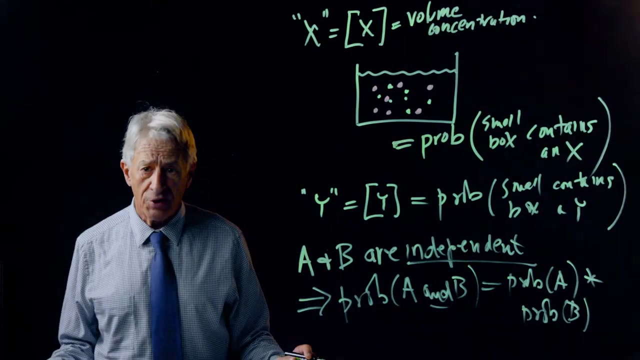 So the probability of drawing a red queen is equal to the probability of drawing a red card, which is 50% times the probability of drawing a queen, which is 13%. So the probability of drawing a red queen is the probability of drawing a queen. 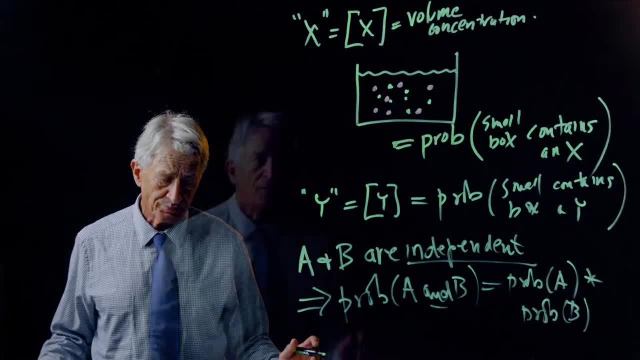 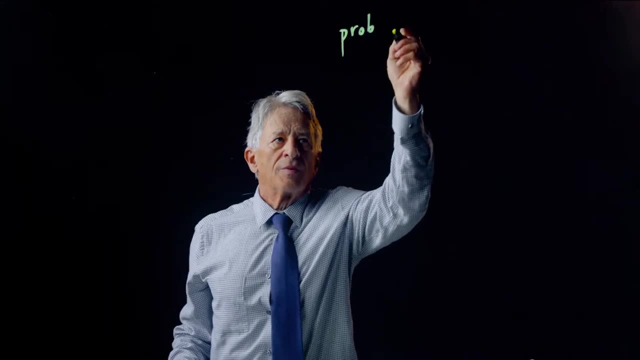 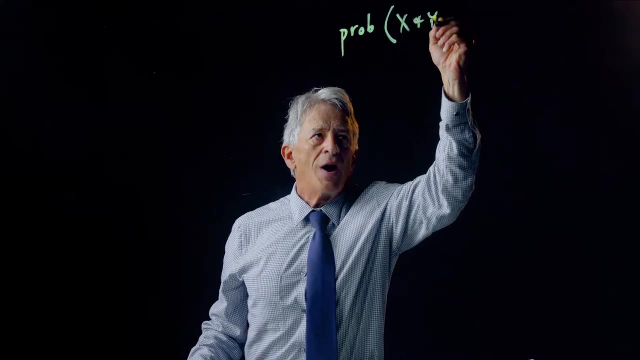 And this is the end product of the two of those, or 6.5%. So we know that the probability- and I'm going to leave out the small box containing the probability of finding x and y is equal to the probability of finding x. 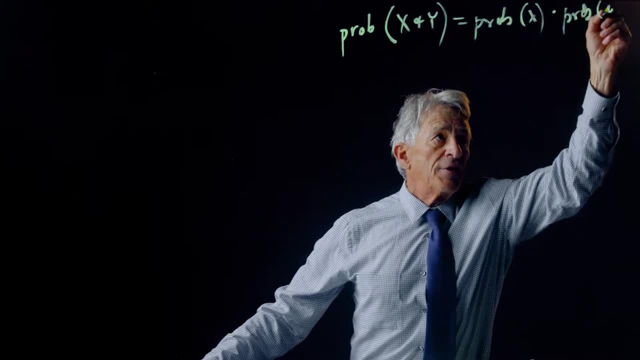 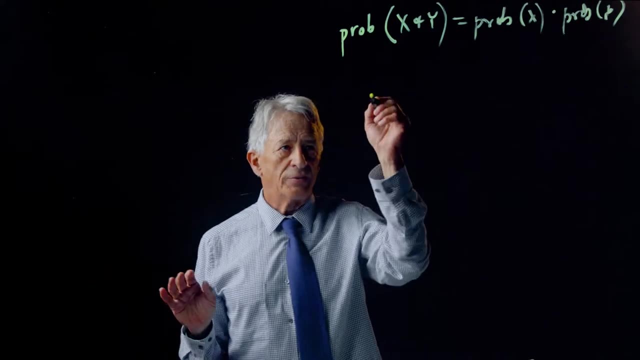 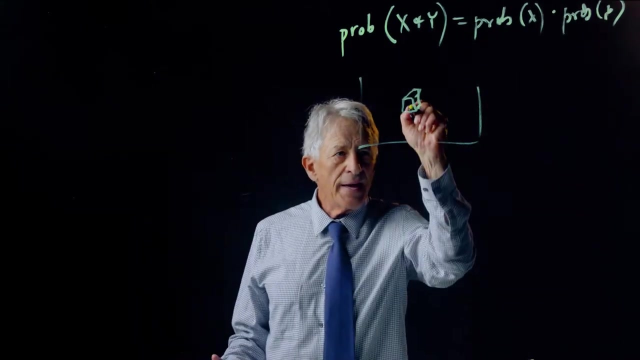 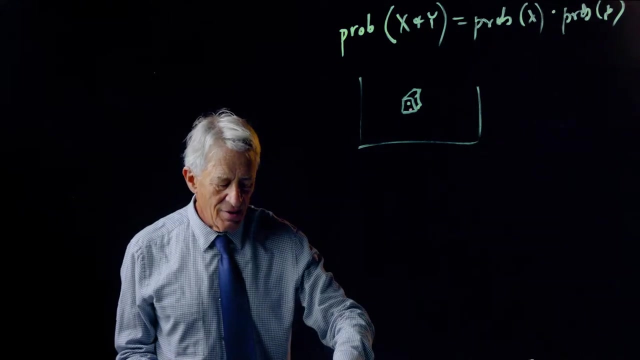 times the probability of finding y. So this is the probability of finding y. And then Now suppose we're in this little box in the middle of the beaker and we have an X molecule and a Y molecule in that little box. 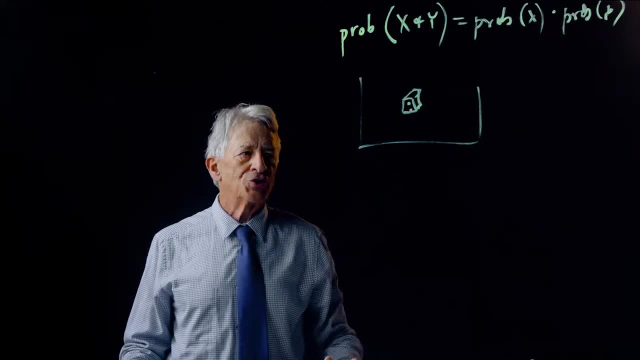 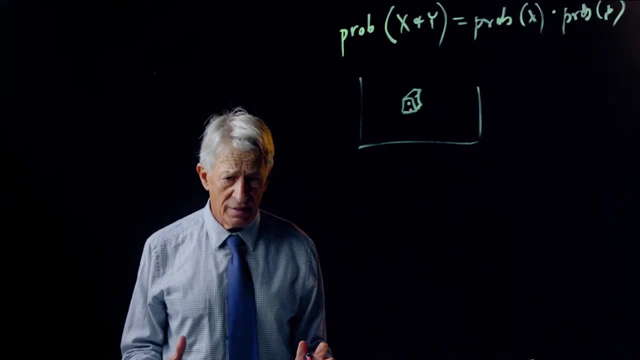 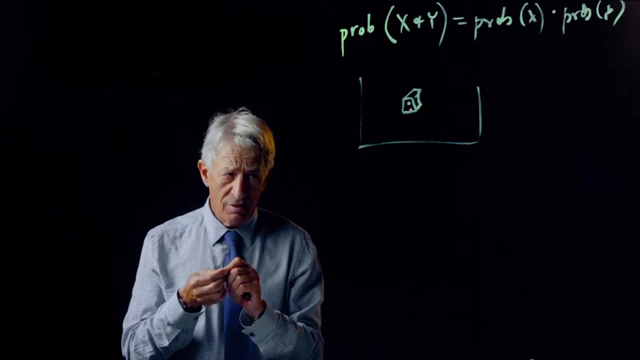 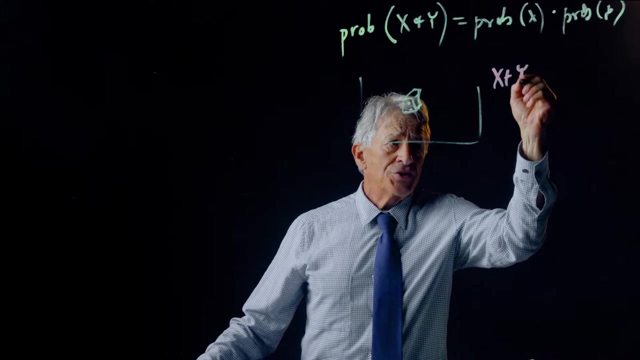 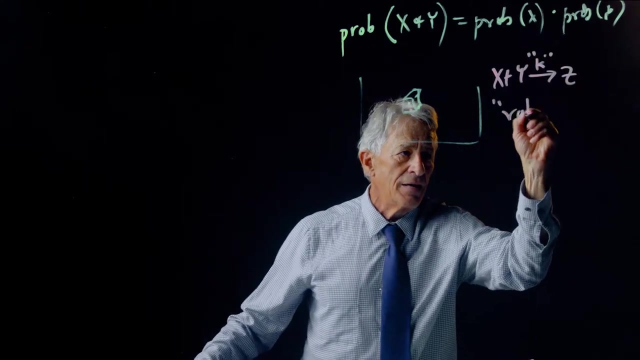 Does it follow that they will chemically combine with each other? And the answer is: not automatically. There is a certain probability that if X and Y are in the same neighborhood as each other, they will actually bind to each other And in the reaction scheme X plus Y goes to Z. with this rate, constant K. 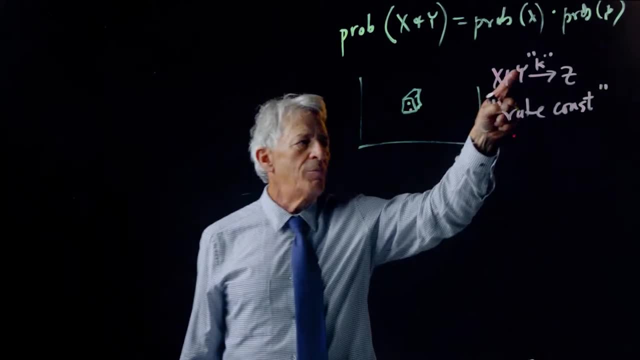 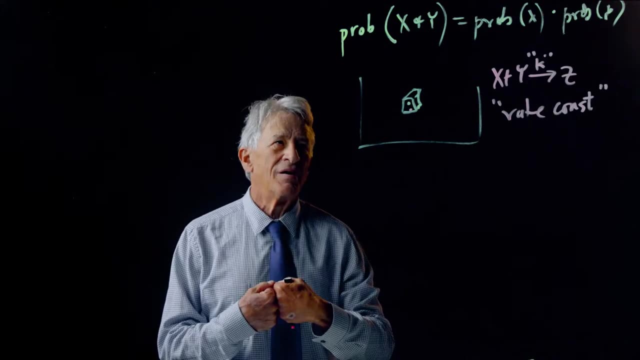 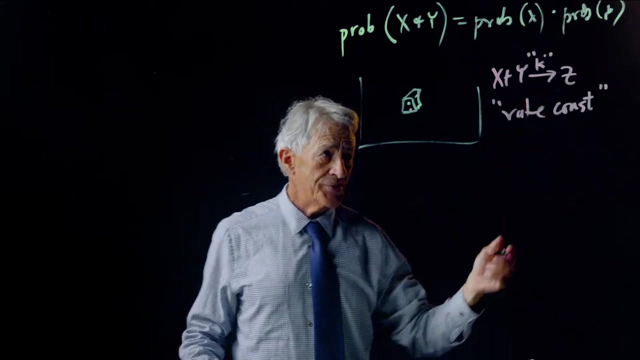 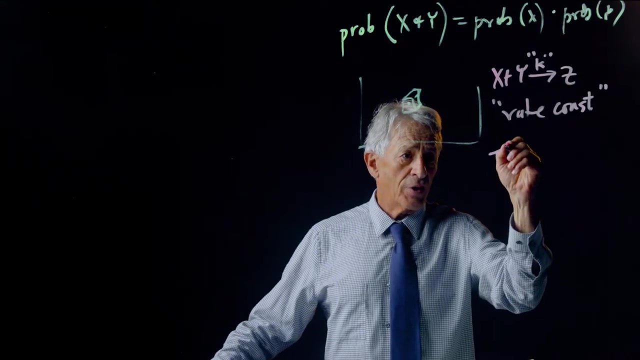 The rate constant is exactly K, The probability that two molecules in a little box will choose to bind together. So the total probability of X plus Y goes to Z is therefore: how much is subtracted from X is therefore clearly minus X times Y times K. 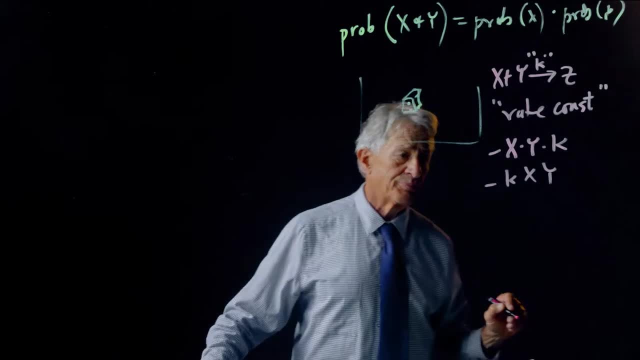 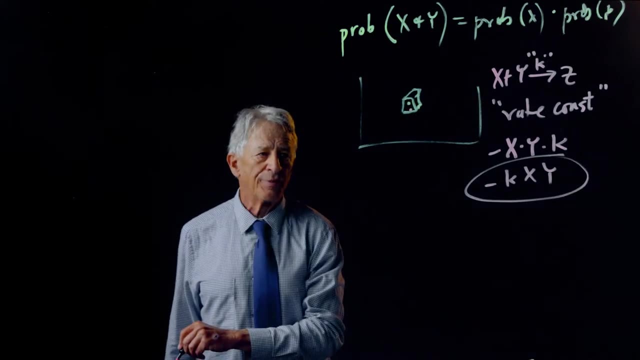 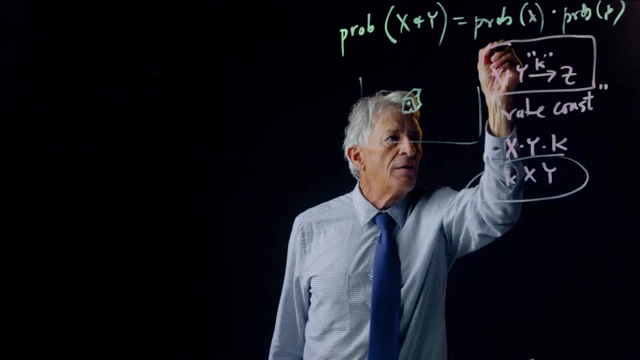 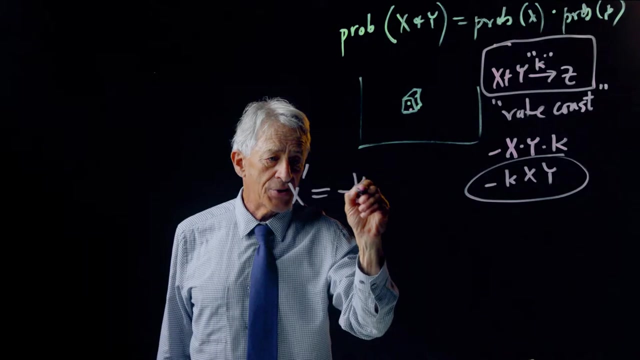 So this is the equation that we usually put in minus Kxy. So now, with this observation, here is our X combines with Y terms. So now we can write the full differential equation For this specific rate scheme. we can write it as: X prime equals minus Kxy. 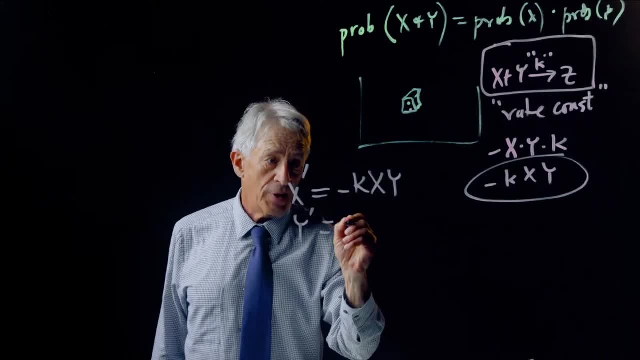 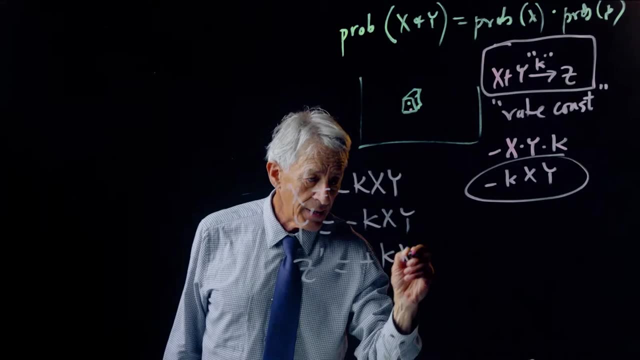 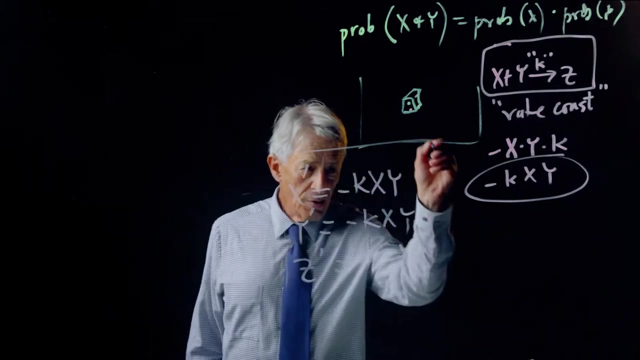 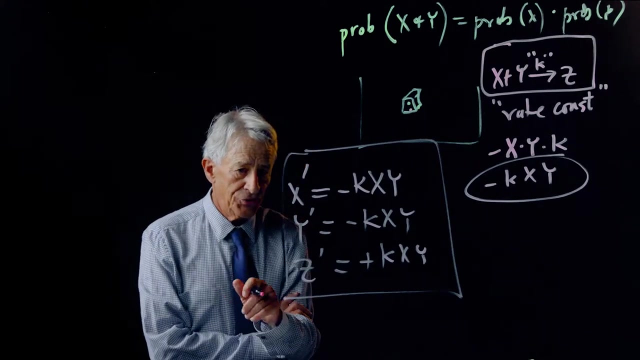 Y prime equals minus Kxy. So we're going to subtract Right minus k x, y and z prime equals plus k x, y And we set initial conditions and this will determine the progress of the chemical reaction. And in this way we have converted the rate. 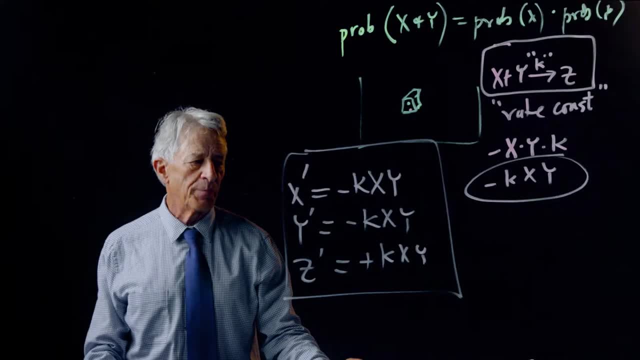 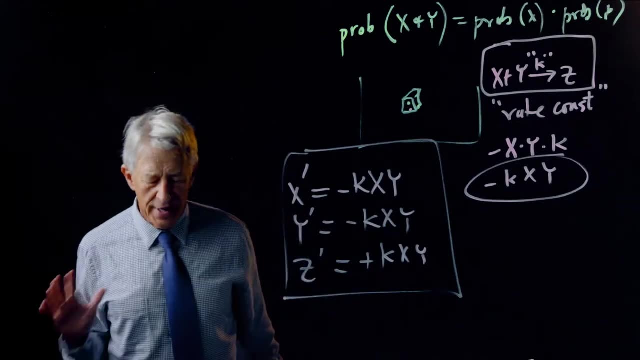 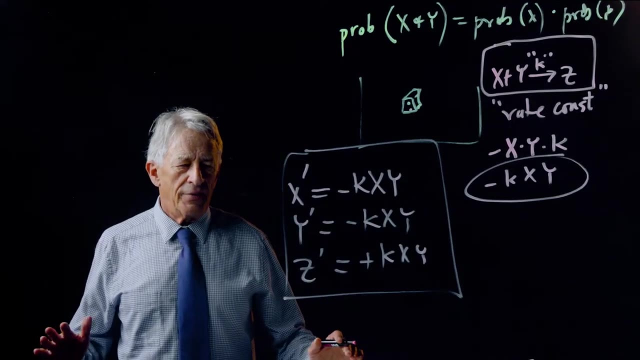 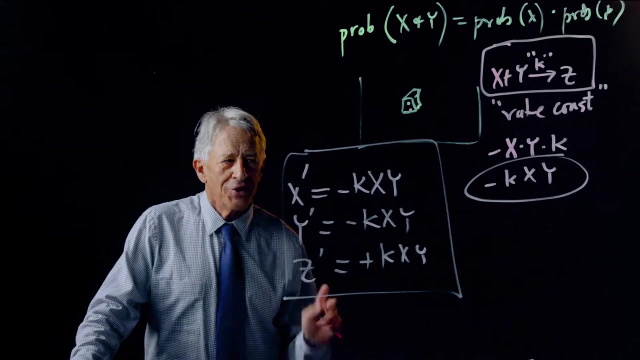 law into a true differential equation. Now, in so doing, you may have heard overtones and analogies to what we said about sharks and tuna, And the answer is: the analogy is a hundred percent. We use the phrase chemical species to talk about sodium and chloride. 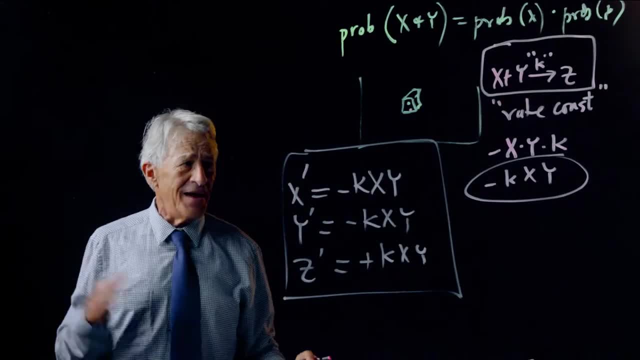 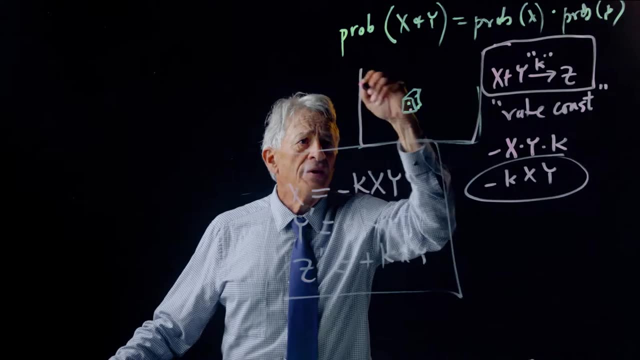 and iodine. We use the phrase chemical species to talk about sodium and chloride and iodine going to sodium chloride. We call those chemical species And they're exactly like animal species And so the simple law here that says that we have a lot of x's and a lot of y's. 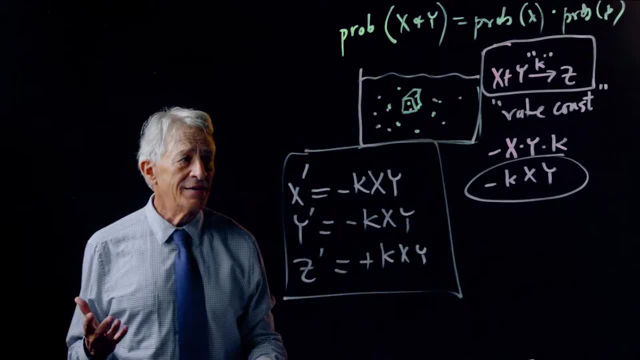 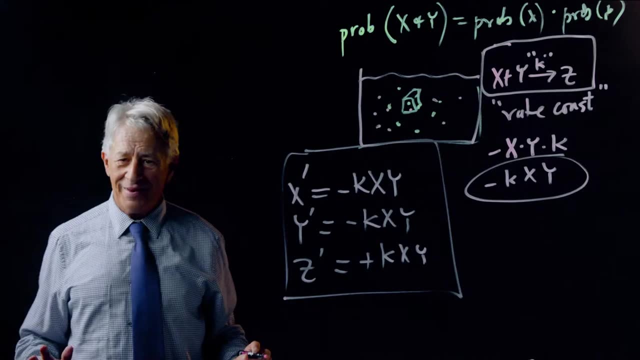 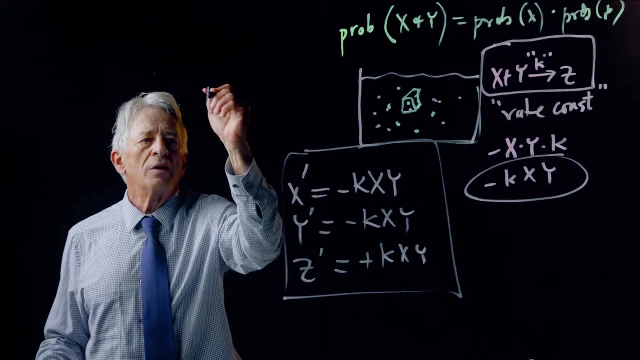 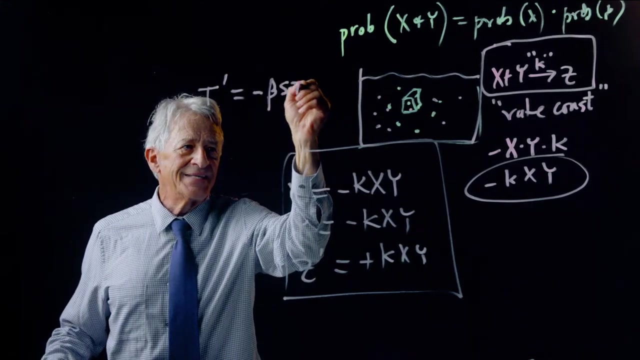 and they bump into each other or not. and when they do bump into each other, they have a probability k of meeting. why? that's exactly sharks and tuna, And you remember the term in the tuna prime equation? that was minus beta s t. 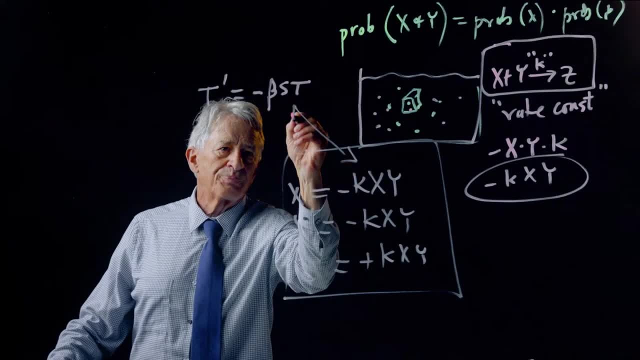 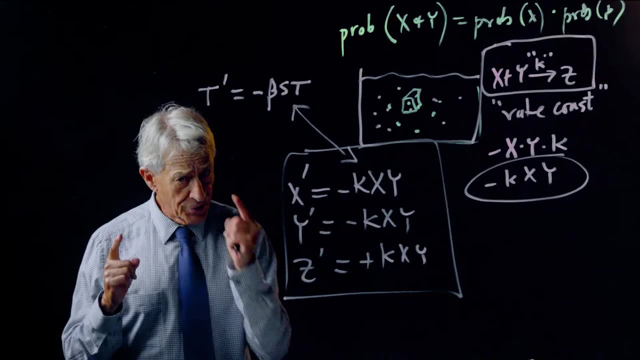 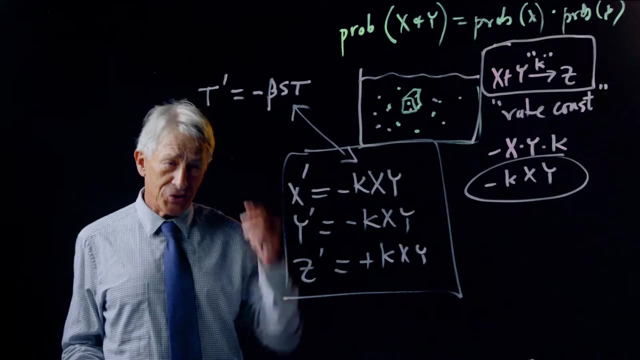 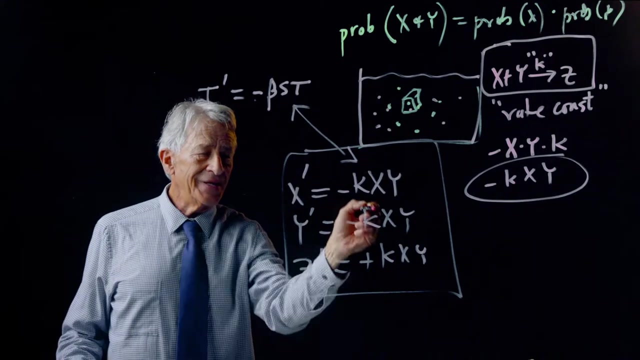 Well, that is this term. And what was beta? Beta was the likelihood that a shark-tuna interaction results in a binding, that is, in the coupling of the shark and the tuna to the detriment of the tuna. But the model is the same. 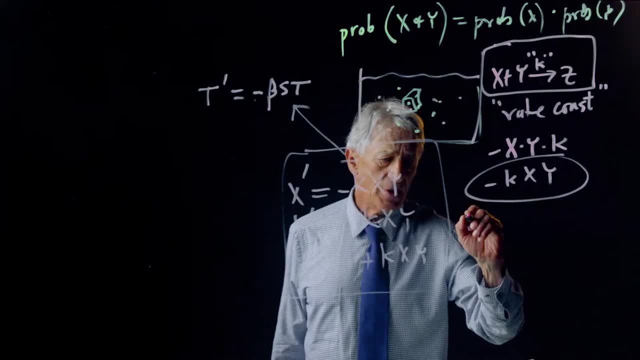 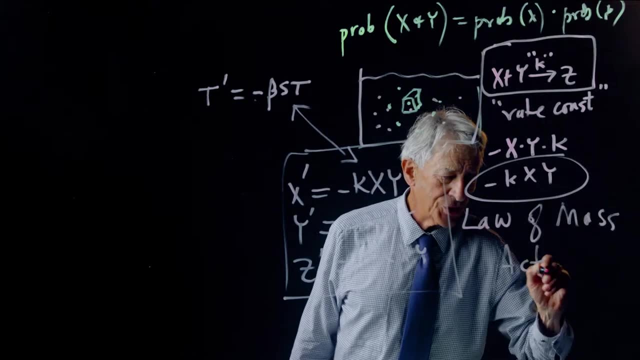 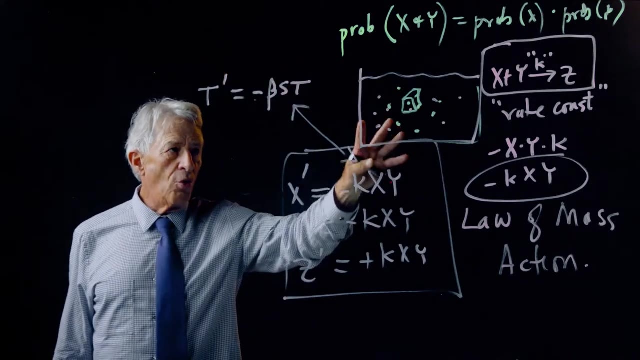 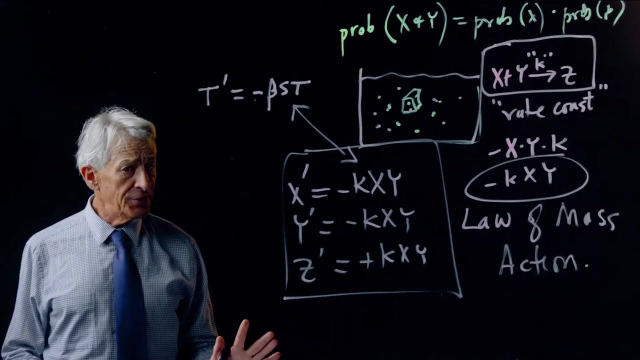 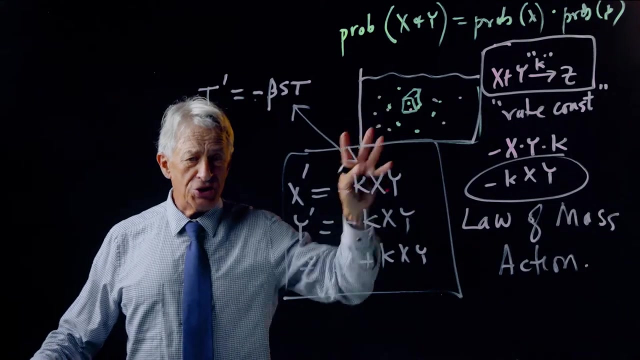 And they're both based upon what in chemistry is called the law of mass action, which says basically that all of the species here- x and y and z- are independent of each other. In particular, it cannot be the case that the solution is so dense, is so crowded. 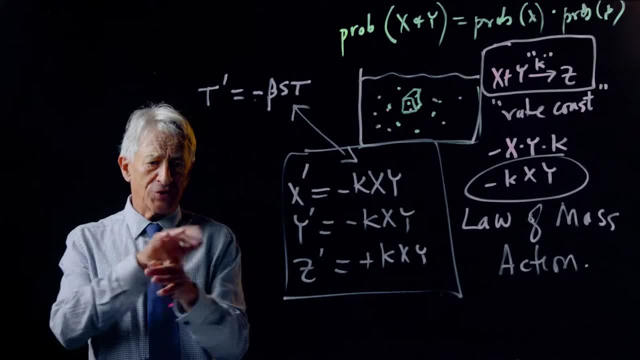 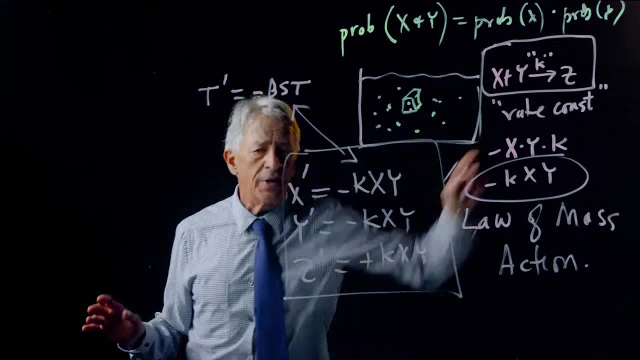 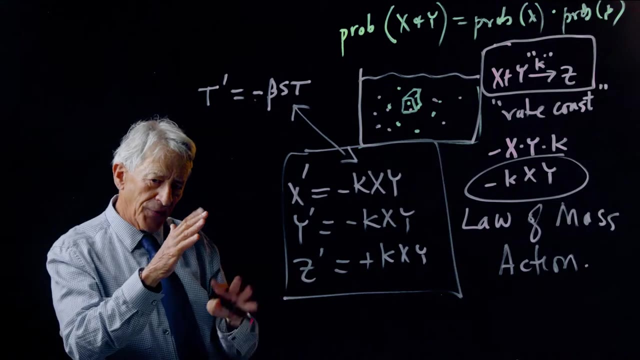 that the x's and y's can't freely diffuse with respect to each other. Because if they can't freely diffuse with respect to each other, then the probability argument breaks down. Because if the x's can form a little wall and wall off the y's so that they can't diffuse, 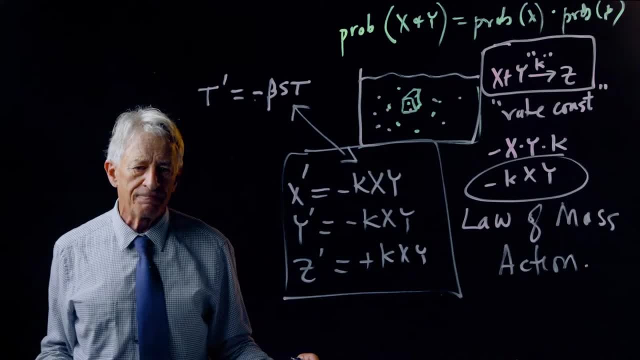 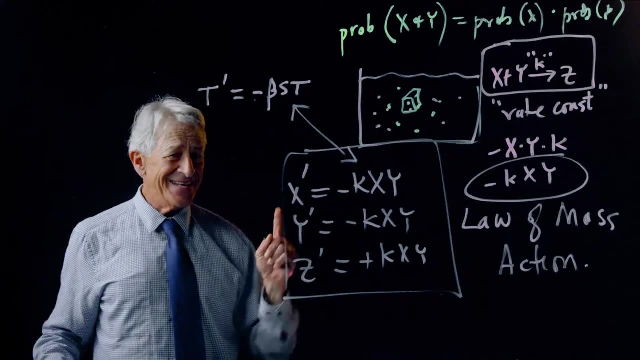 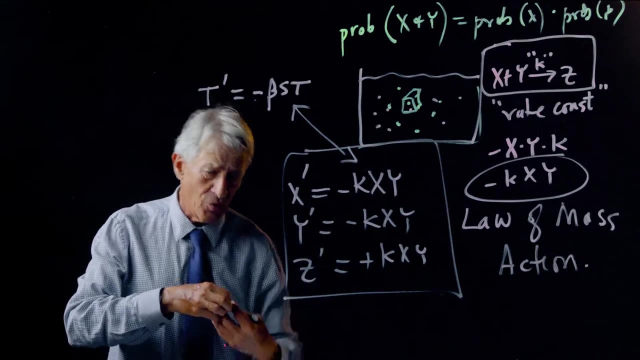 through the fluid, then the whole probability argument breaks down. So we're assuming that x is independent from y, that they're both dilute enough that there's no crowding effect of the x's with themselves or the x's with the y's. 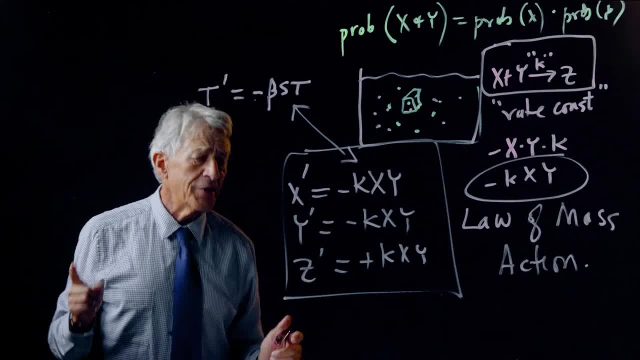 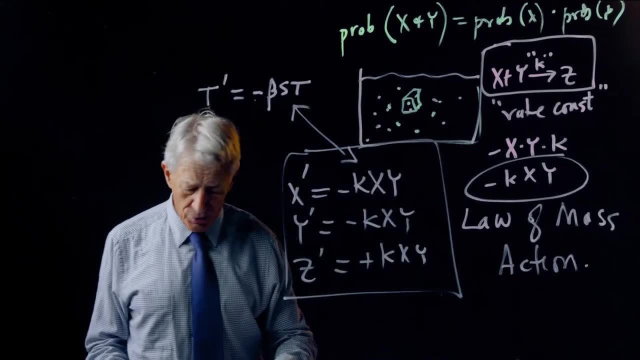 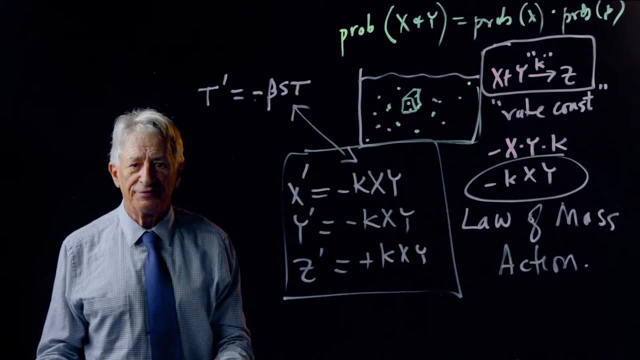 or the y's with themselves. But it also can't be, or it can't be too dilute, because if it were one X molecule down here and one Y molecule up there, you could wait an awfully long time for them to fall into the same area. 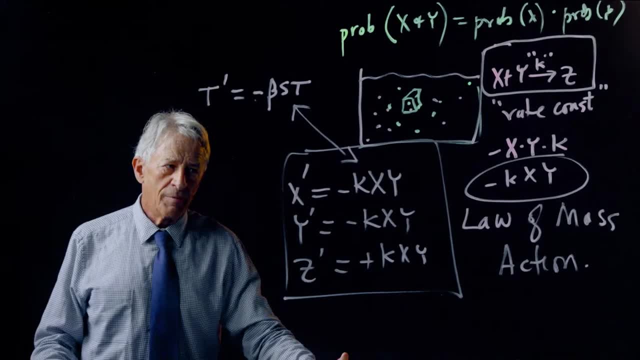 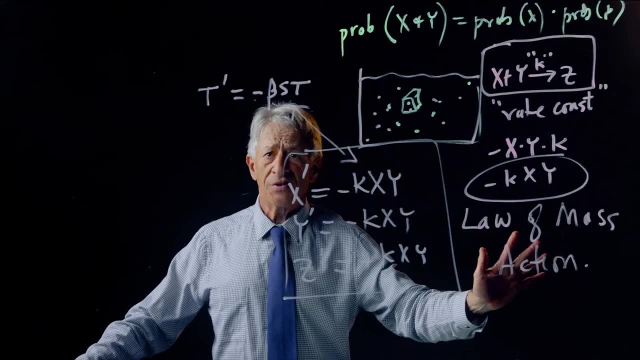 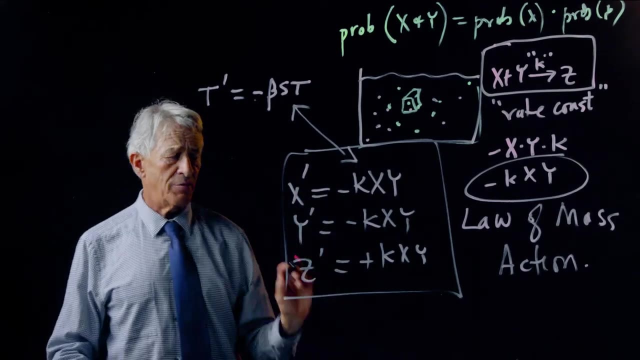 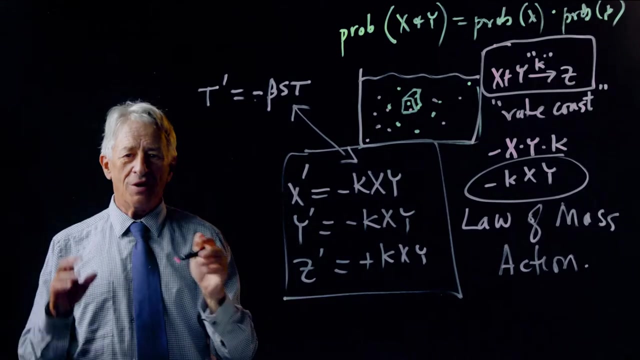 and this argument would also break down. But in that intermediate range of not too dilute and not too concentrated, the law of mass action applies and it is essentially the same as shark-tuna dynamics. In fact, you can write the shark-tuna scenario. 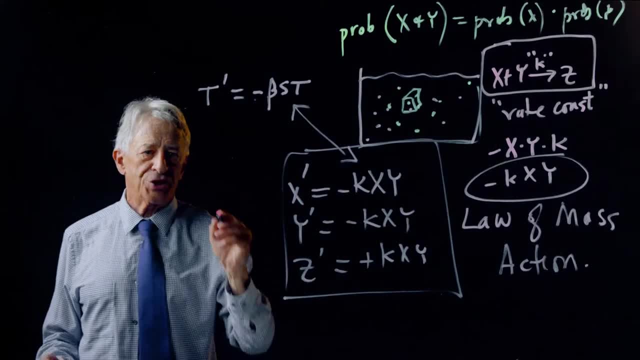 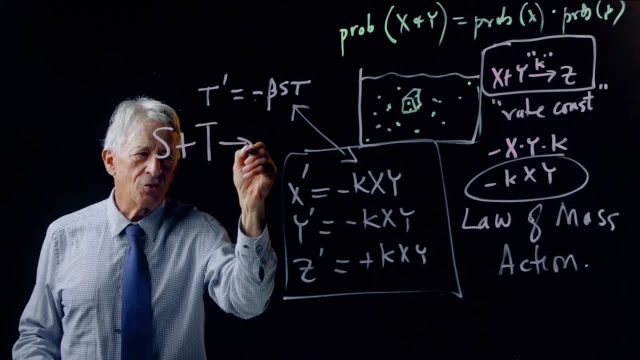 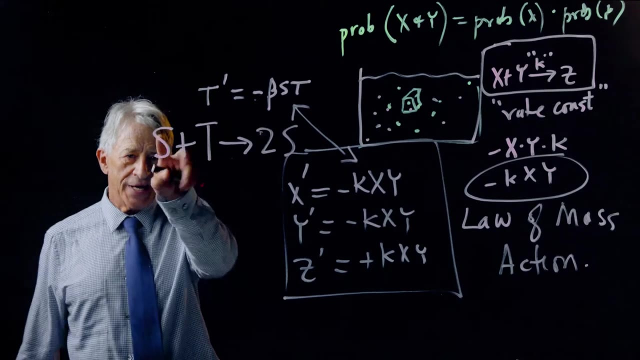 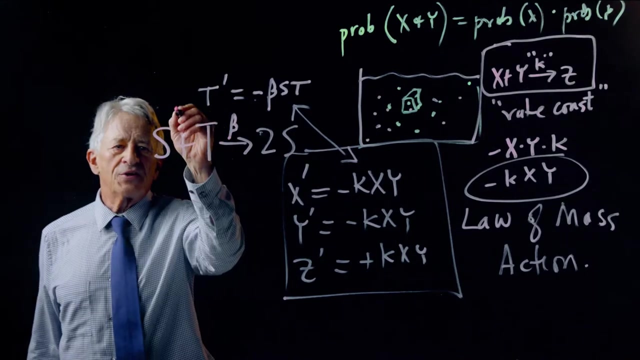 as a goes-to reaction. For example, you can write S plus T goes to 2S And that is a reaction in which S and T combine and, of course, the K. there is going to be beta. So what does this rate law say? 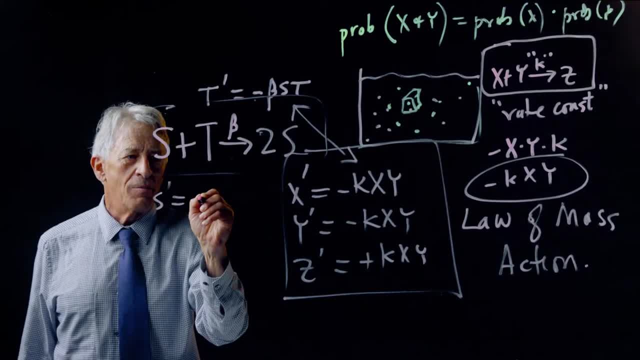 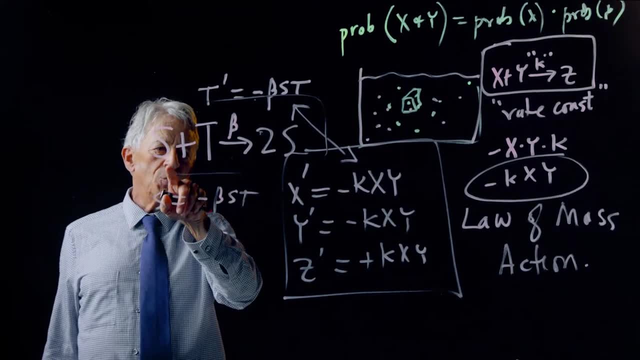 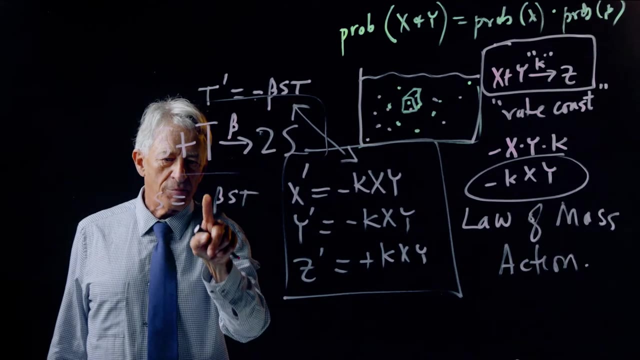 It says that S prime equals minus beta S T, because you are going to lose a shark here and gain 2 over that There, so I'm sorry that should be a plus, not a minus. Shark prime is equal to beta S T. 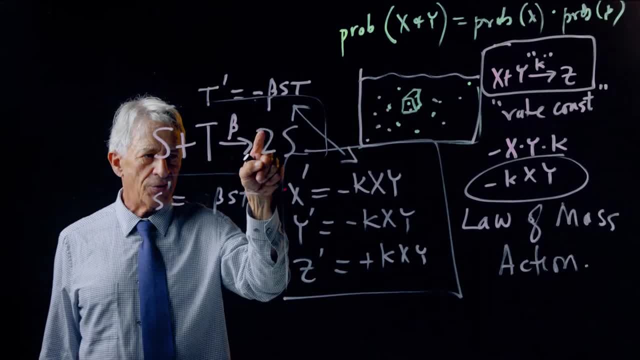 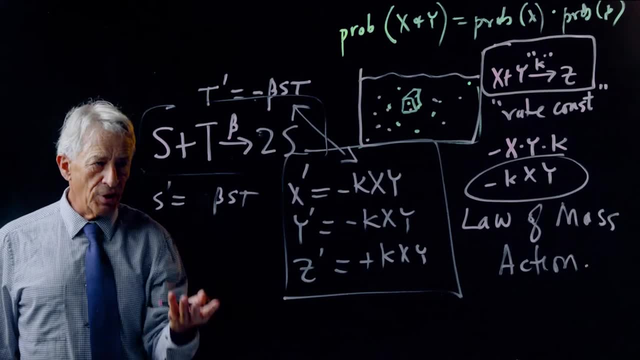 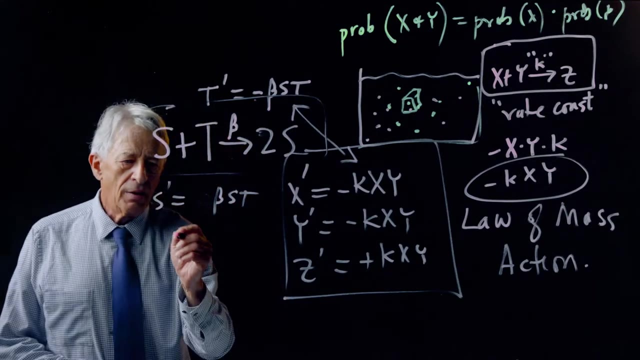 because you lose a shark from the left, you gain 2 sharks on the right. That's a net gain of a shark at a rate. beta, S, T And similarly the other terms of the shark-tuna model. I wrote them down. 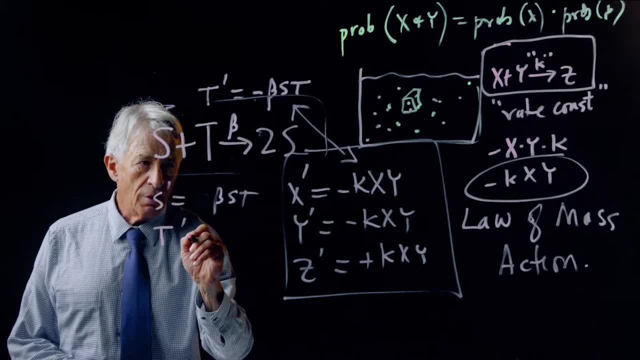 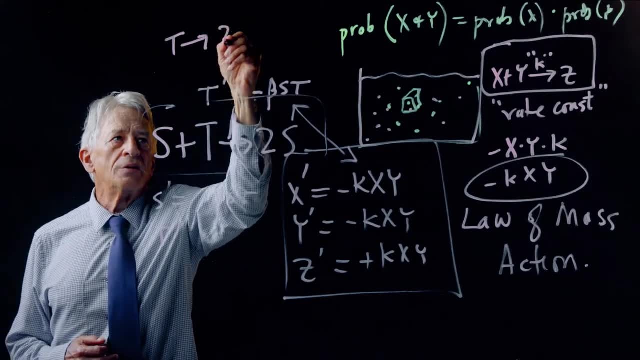 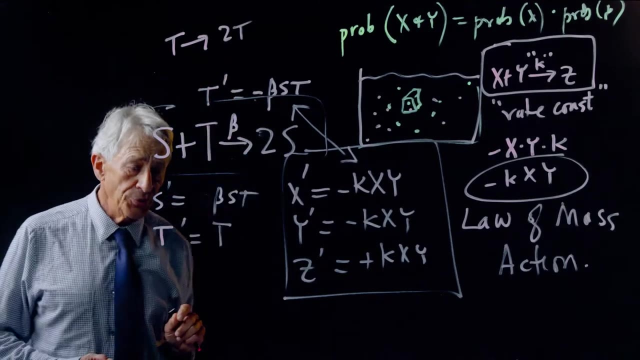 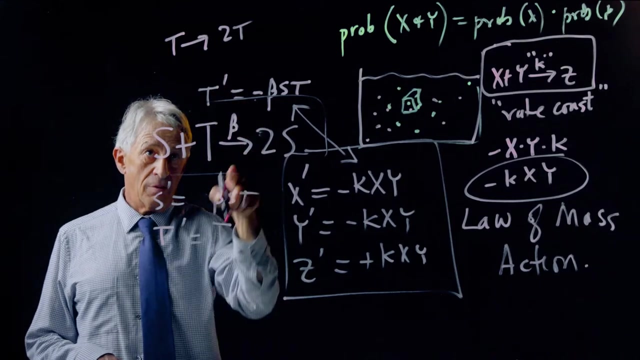 Now we have to write the tuna expression and we can write T. Let me write it over here: T goes to 2T, So that says that T prime equals T. You lose one, you gain two. But T prime also equals minus beta S, T. 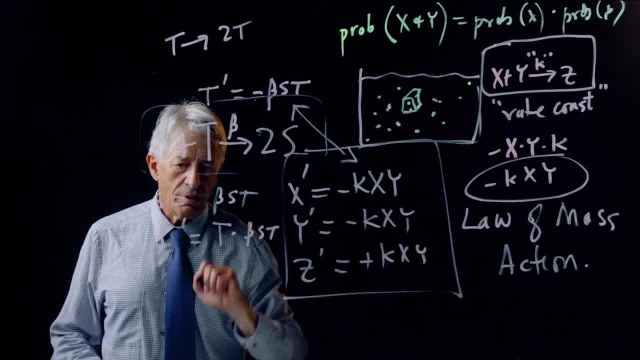 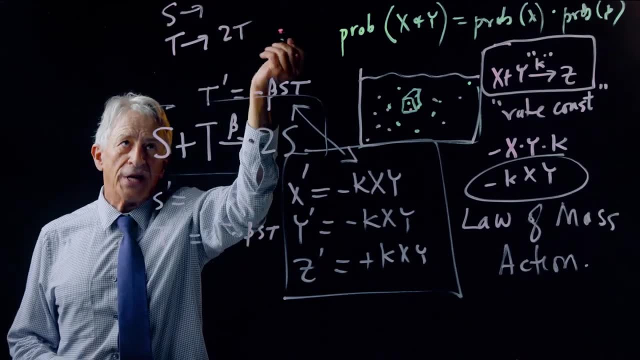 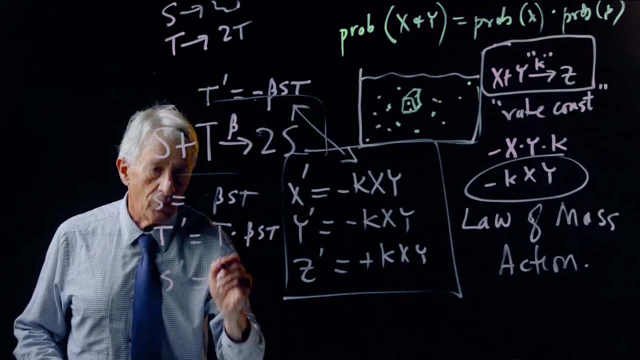 in our differential equation And we can write: T prime equals minus beta, S, T. And then, lastly, the last rate law we need is: shark goes to dead shark, or shark just goes to the cloud, And that's of course gonna be S prime equals. 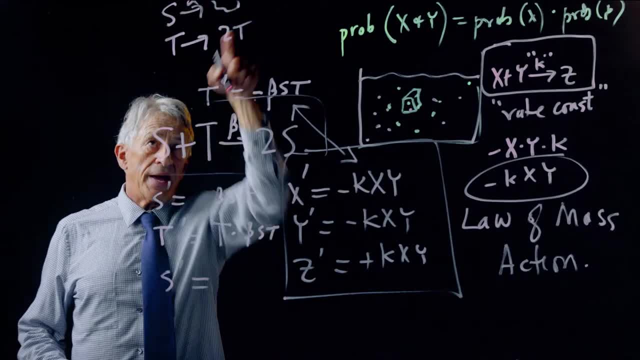 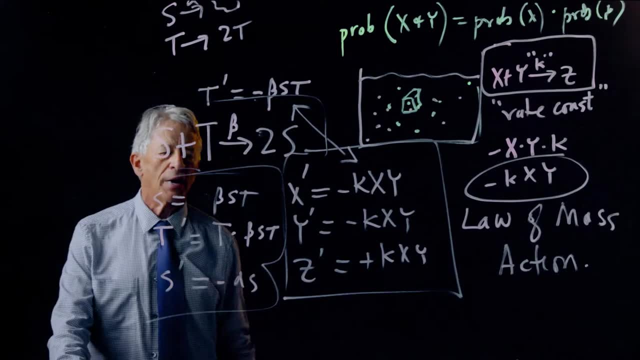 and this is a death rate D, And so that is going to be minus D, S, And if we add up these terms we get the shark-tuna model. So the shark-tuna model and the chemical species meet and bind with each other. 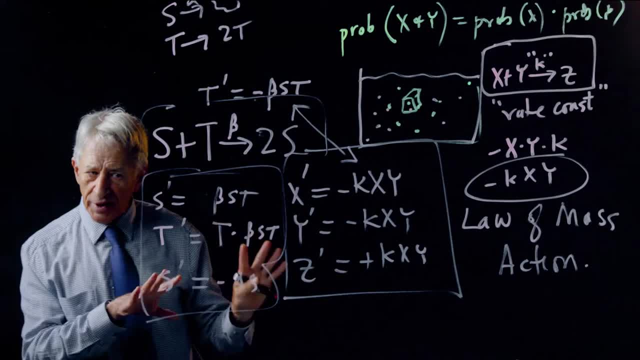 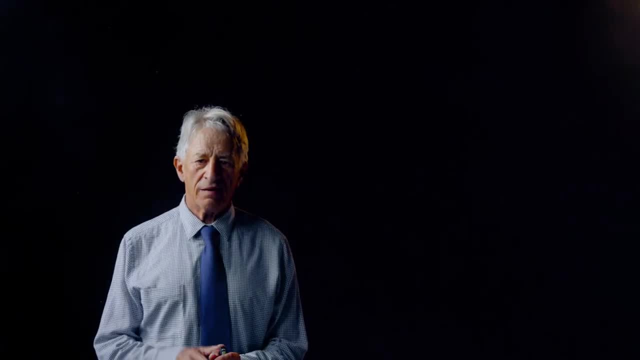 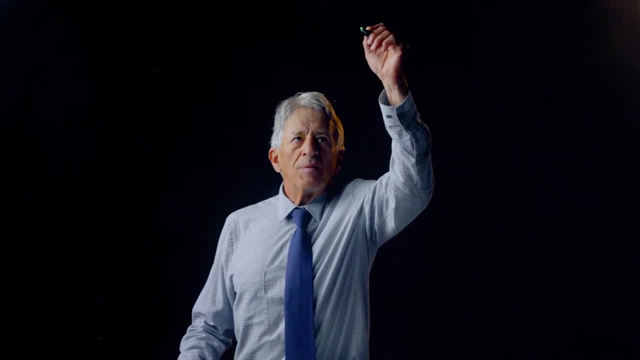 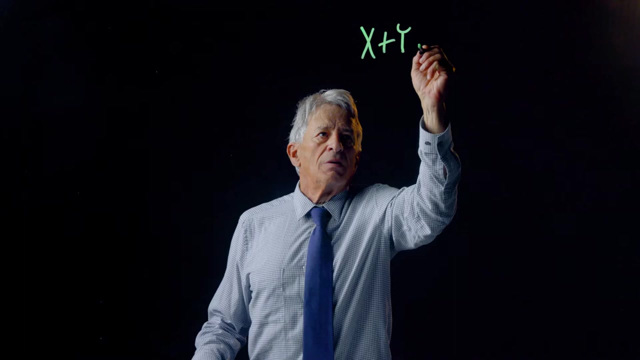 is exactly the same underlying dynamics And it gives exactly the same type of differential equation. So that's how to take X plus Y goes to Z and turn it into a differential equation. Let's take a little bit more complicated example now. Let's include a back reaction. 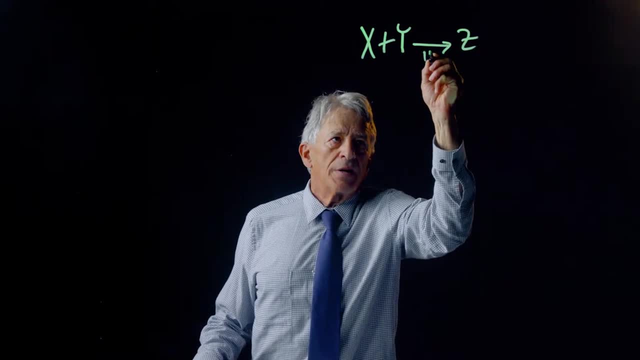 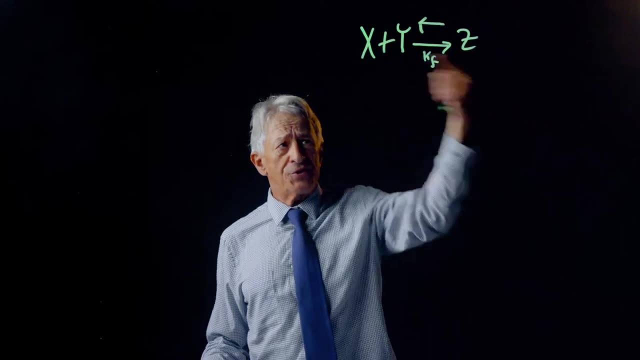 So X plus Y is gonna go to Z and the K there is gonna be is gonna be K forward, And then Z is going to dissociate back into X and Y And that is at a rate constant, with a rate constant of KB. 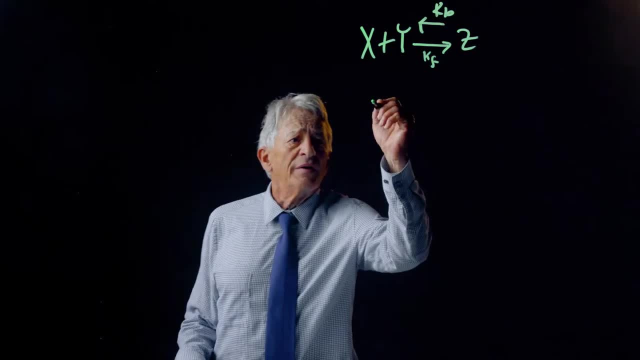 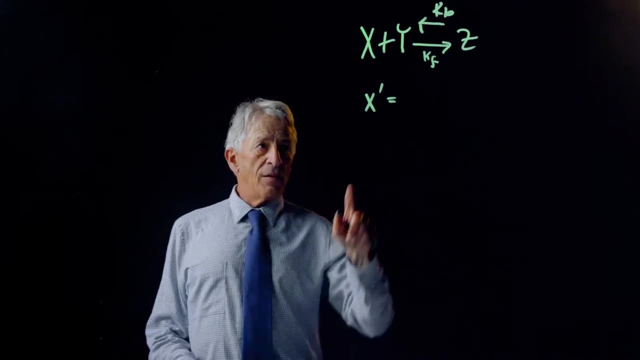 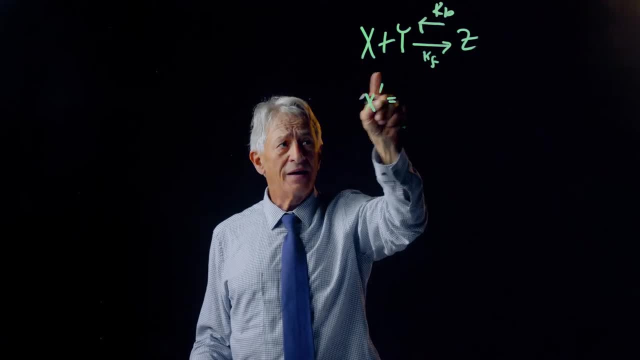 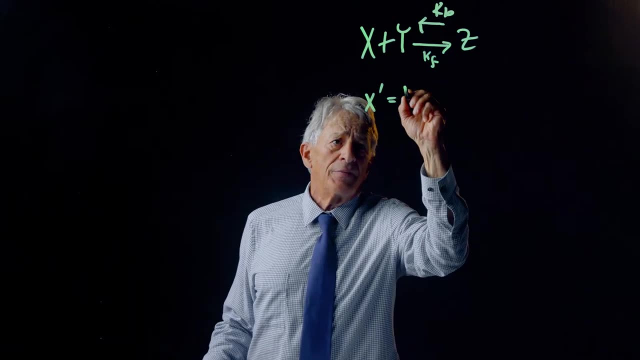 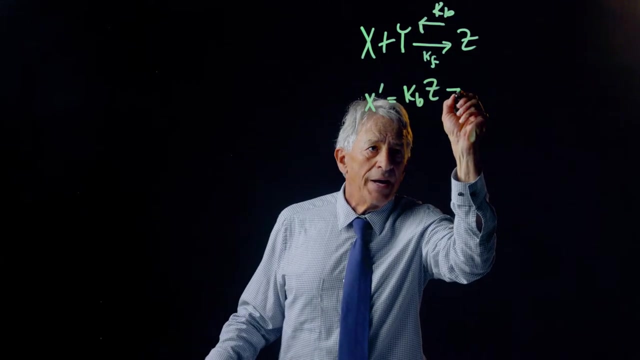 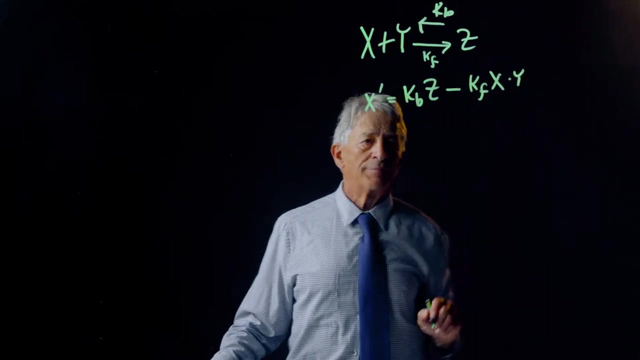 of Z into X and Y And that takes place at a rate KB. So now we have a plus term here And that plus term is KB times Z. Same minus term for the forward reaction, which is K, forward times X times Y. 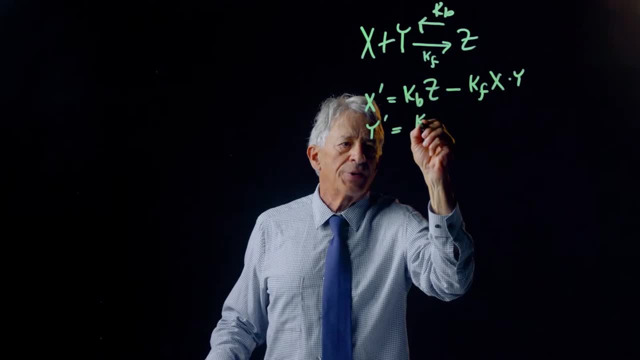 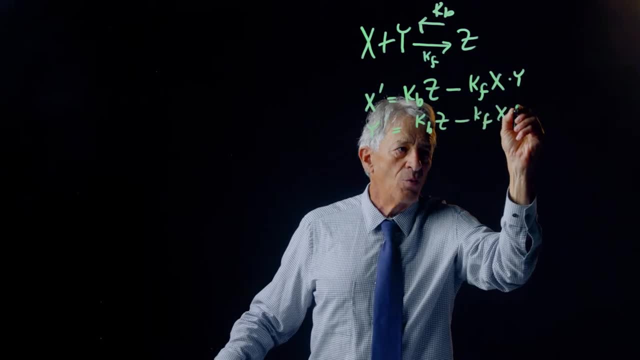 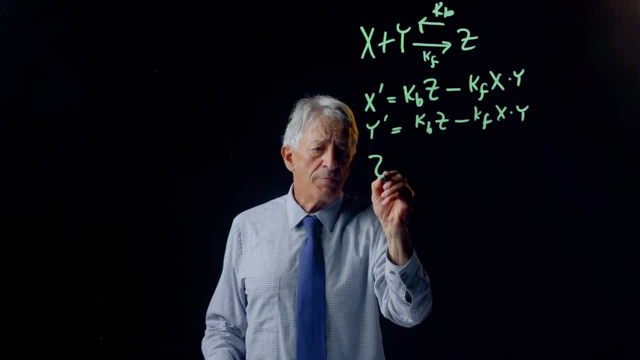 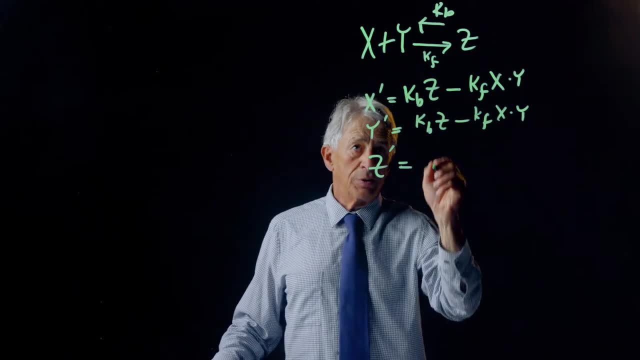 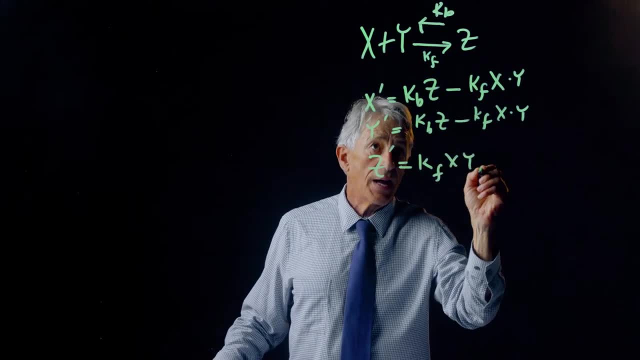 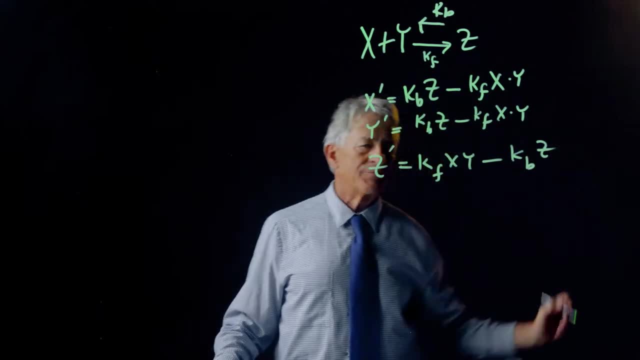 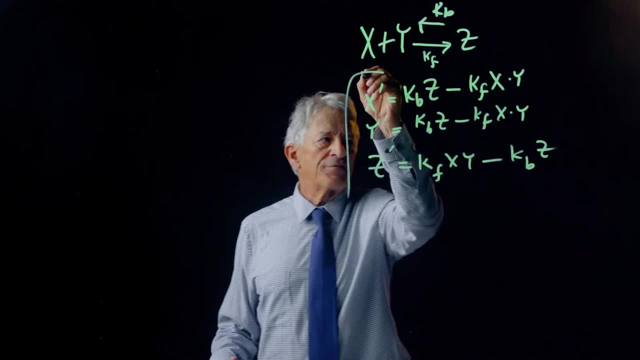 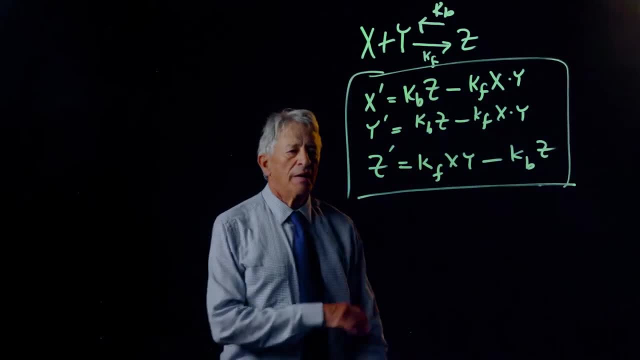 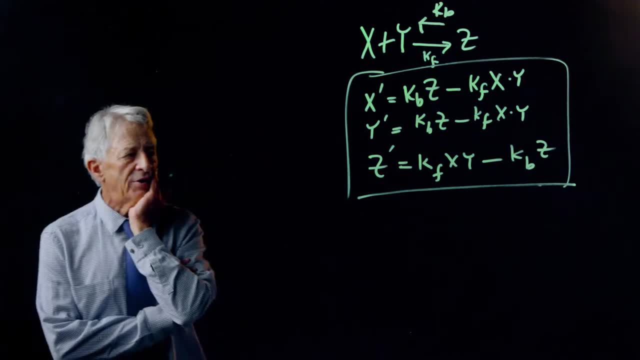 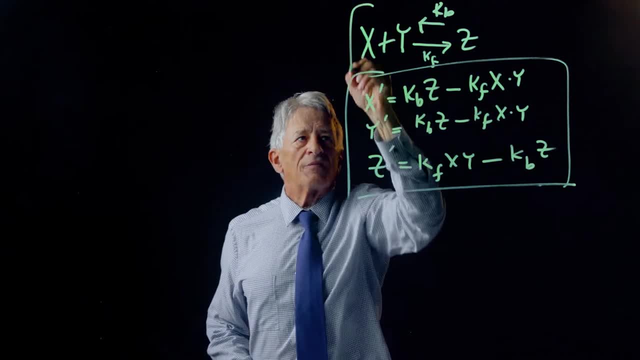 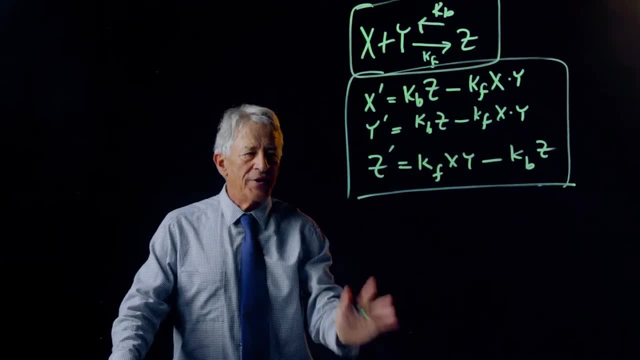 Similarly, Y prime is equal to K forward times X times Y. Similarly, Y prime is equal to Y forward times X times Y. Similarly, Y prime is equal to K forward times X times Y. Similarly, Y prime is equal to K forward times X times Y. 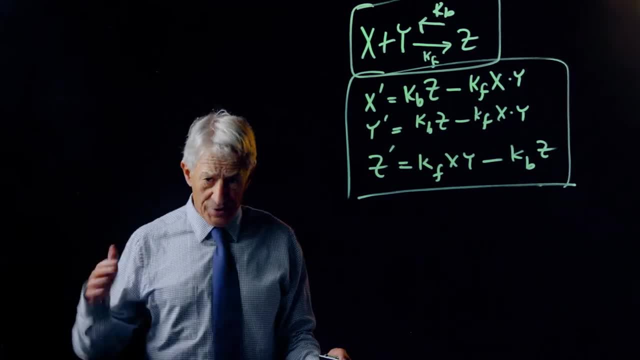 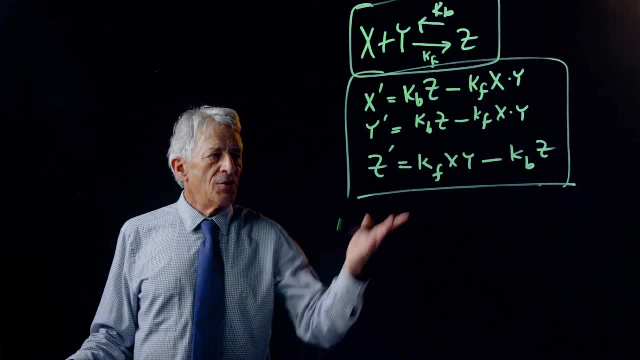 Similarly, Y prime is equal to K forward times X times Y. The answerror isанию gdg. The answer is we can. so a very simple and very cool thing. This anticipates really what our next big dynamics subject is. This is a differential equation model. 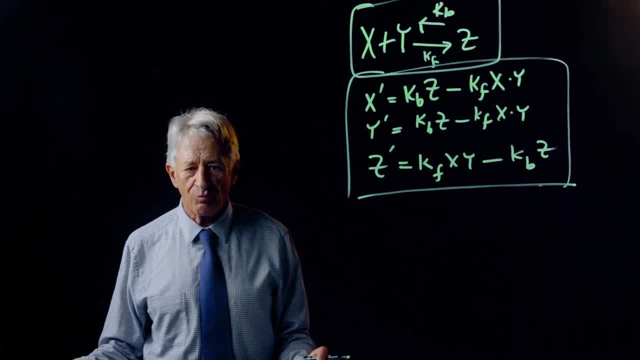 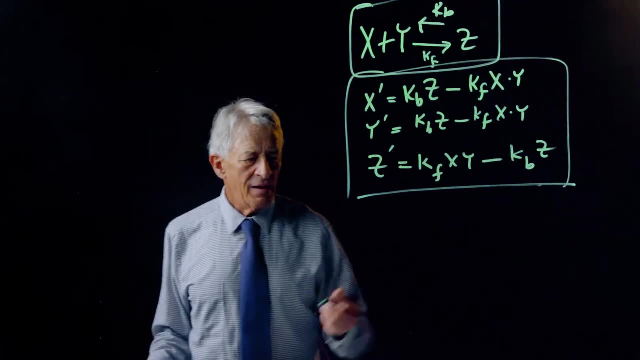 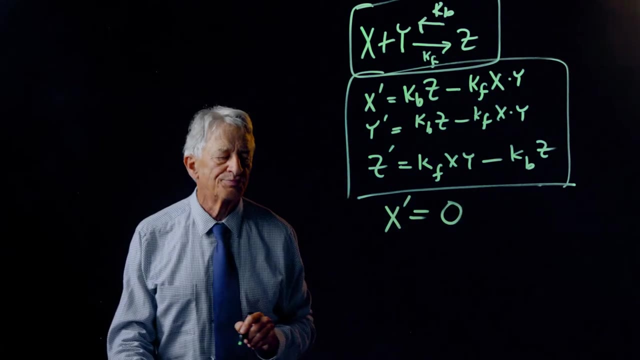 It is going to predict some kind of trajectory. We do not offhand know what it is. We can make one observation. We can make one observation. I want to think of the very special case, Click, in which x prime equals zero, which is also known as equilibrium. 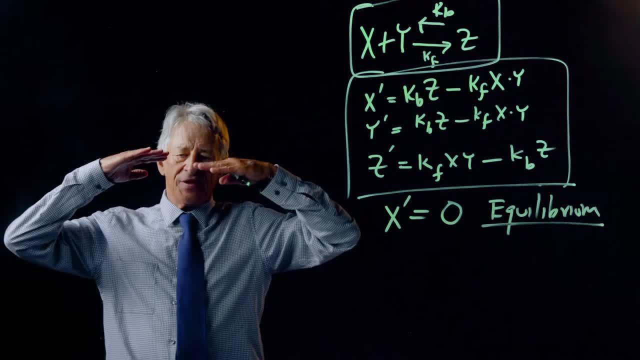 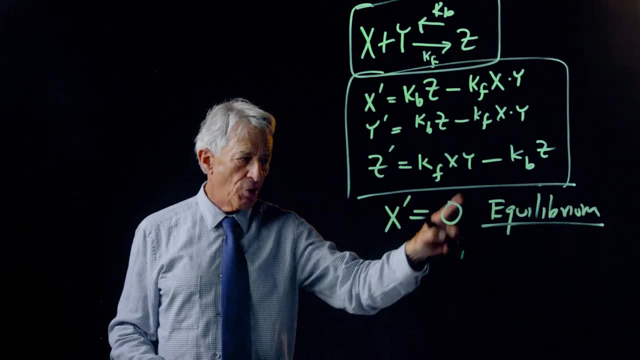 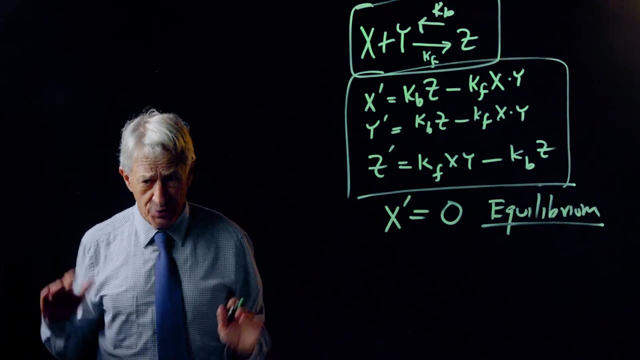 So at chemical equilibrium these quantities are not changing grossly, And so x prime equals zero and it is said to be in chemical equilibrium, And we're going to be studying equilibrium points of differential equations. a huge subject, but this is our first example of one. 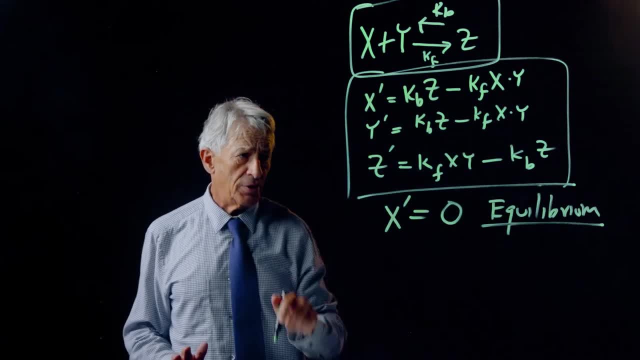 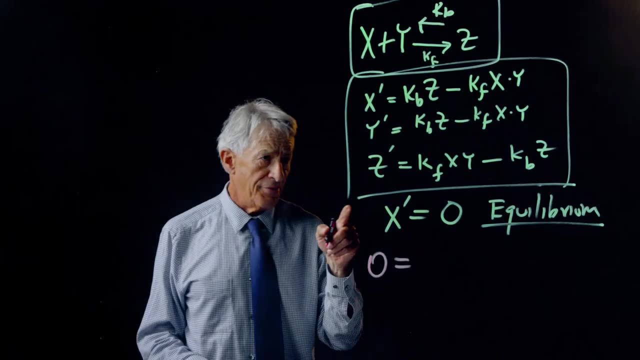 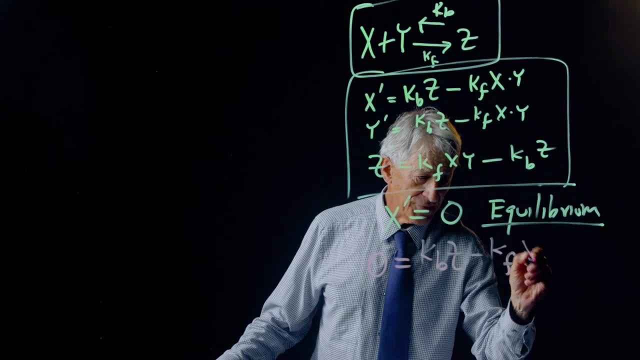 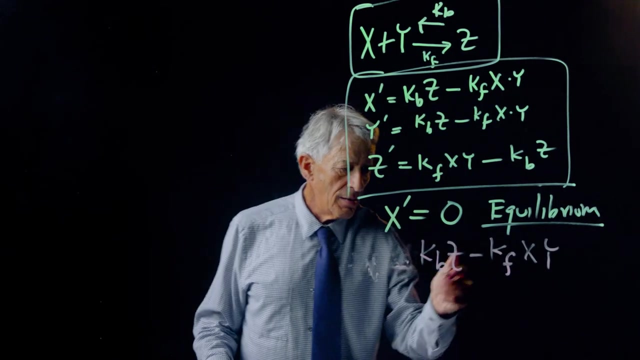 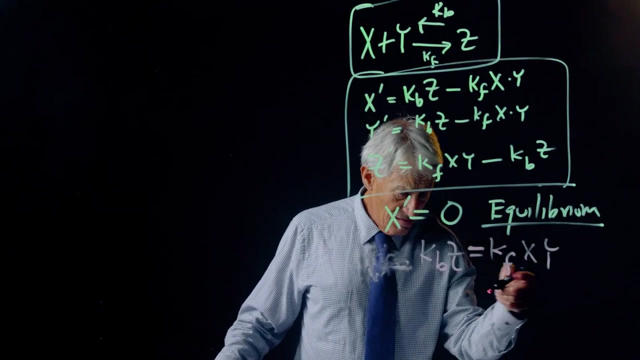 And we can just stare at the top line there and say: well, if x prime is zero, then zero equals kb times z minus kf times xy. Let's drop that, make those two equal. Let's divide both sides by z and divide both sides by k forward.